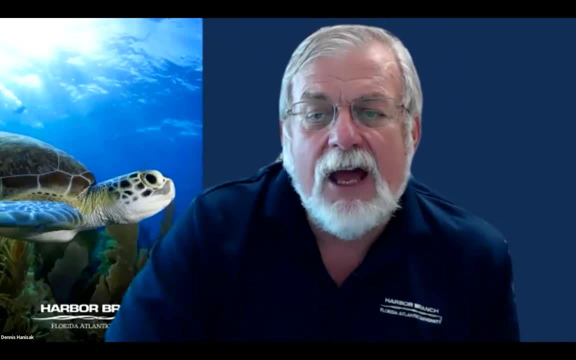 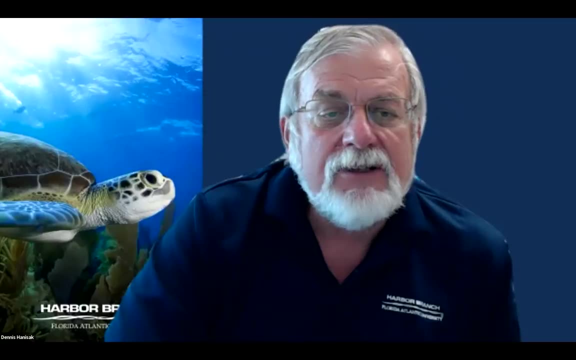 Well, hello, Welcome to today's lecture by Donna Kosak. I'm Dennis Hanusak, a research professor here at Harbor Branch and the host of the series. Our next monthly virtual lecture will be on May 5th at 4 pm. The lecture is entitled Wonders of Greenland- Holy Giant Iceberg. 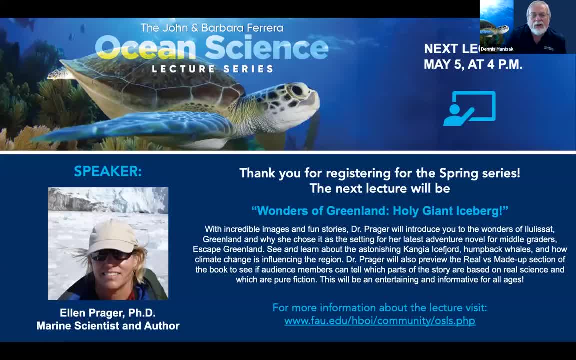 And it will be given by Dr Ellen Prager. She's a well-known marine scientist and author and she's one of our most popular lecturers in the series. And Ellen will introduce us to the wonders of Greenland and why she chose it as a setting for her latest adventure novel for middle graders, which is entitled Escape Greenland. 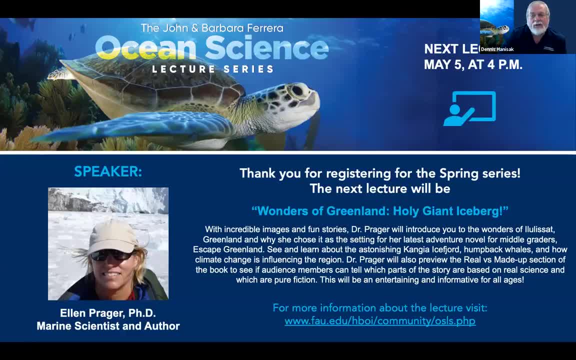 You will learn and see things like the astonishing Kangea Ice Fjord Humpback Whales and also how climate change has influenced the region. Now, some of you may remember Ellen's last lecture was the year before the pandemic started. 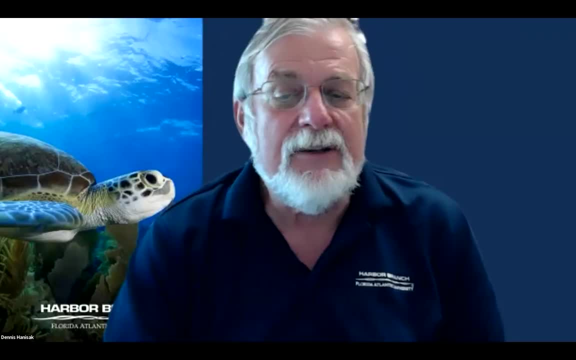 She spoke on the Galapagos, which was the topic of her previous book in that series, And those of you who have heard her speak know that she always has incredible images. She tells very funny and interesting stories. Her lecture will be an entertaining and informative one for all ages. 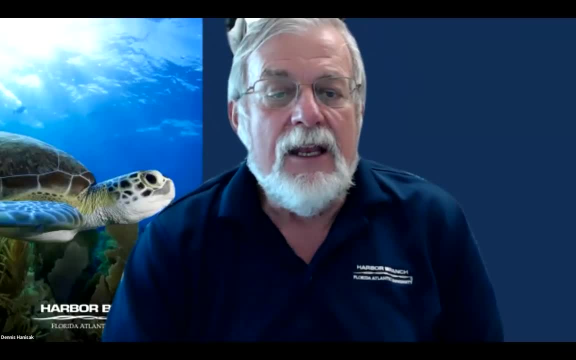 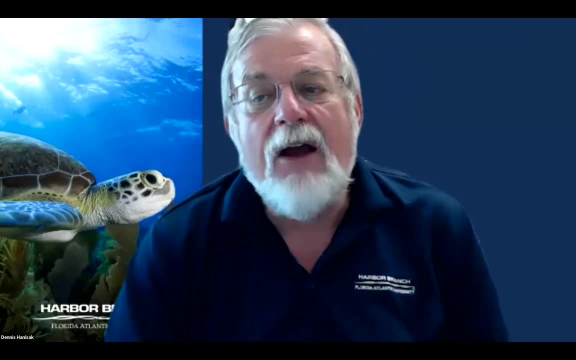 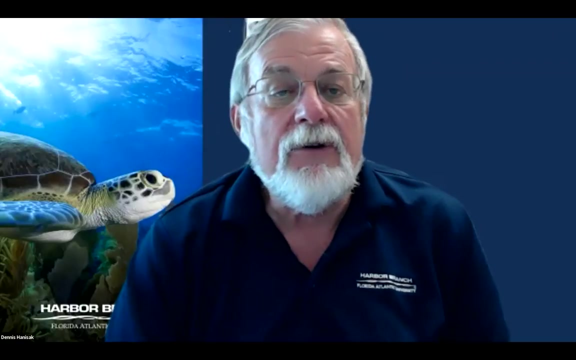 So I really hope that you can join us In May. Now it's my pleasure to introduce today's speaker, Donna Kosak. Donna is an engineering fellow at LE3 Harris, which is up in Melbourne, and past president and UN Ocean Decade liaison for the Marine Technology Society. 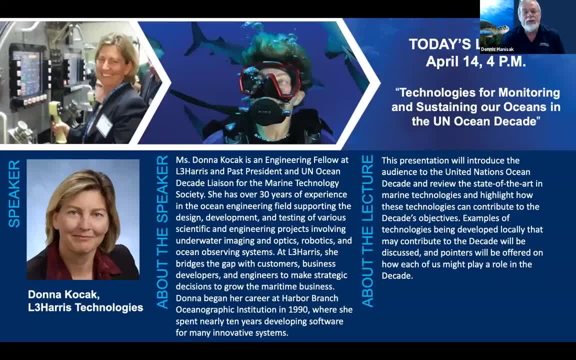 She has over 30 years of experience in the ocean engineering field, supporting the design, development, testing of various scientific and engineering projects involving underwater imaging and optics, robotics and ocean observing systems. At LE3 Harris, she bridges the gap with customers, business developers and engineers to make strategic decisions to grow the maritime business. 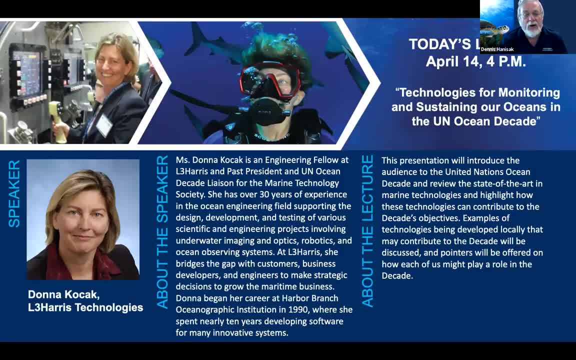 Donna has a bachelor's degree in computer science for the University of Central Florida. She has two master degrees: One is an MBA from the University of Florida and the other is an industrial engineering management at the University of Central Florida. Donna began her career of engineering and engineering at the University of Central Florida. 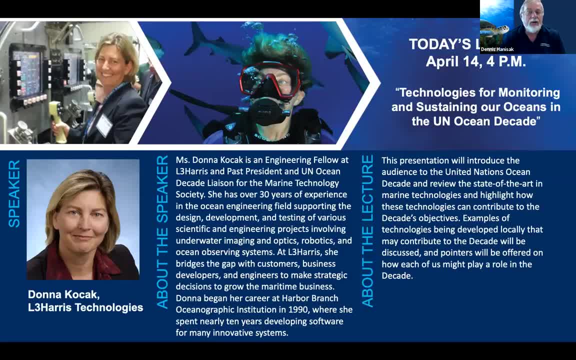 career in what was then our division of ocean engineering at harbor branch in 1990.. uh, so she kind of had her, she kind of started profession to grow up here, so to speak, like some of us have, and she spent 10 years here developing software for many innovative systems. i would be remiss if 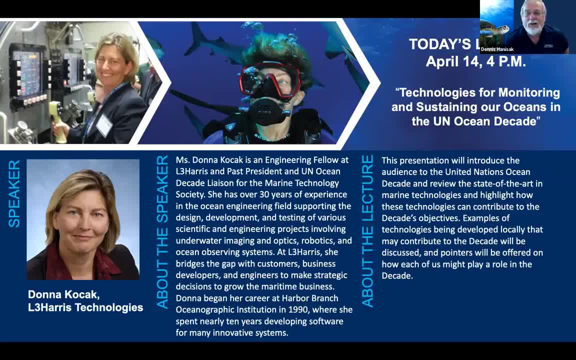 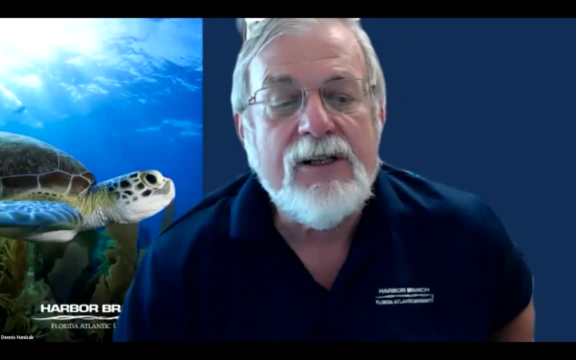 i also didn't point out that she was one of our stars on our famous 1990s uh era harbor branch softball team. so let's welcome donna kosak to our virtual podium for her lecture on technologies for monitoring and sustaining our oceans in the un ocean decade, and it's great to have you back, donna. 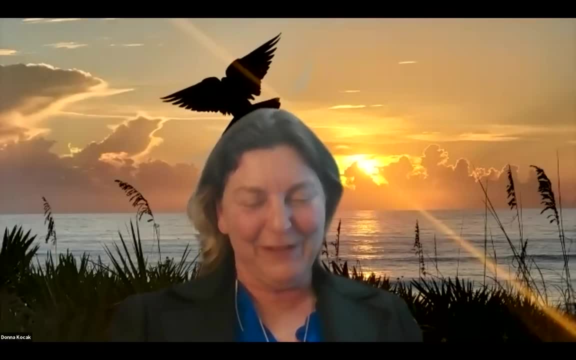 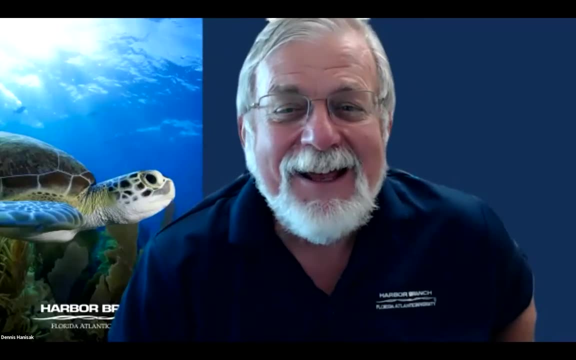 thank you very much, dennis. that was great. um, the softball means a lot to me, although you did forget one of my master's degrees, but that's okay, i i prefer you have another one. i do. can i trade? can i trade them in three of them in for well? i think you can get for three. 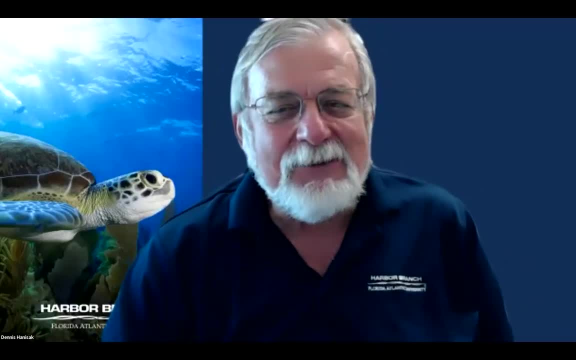 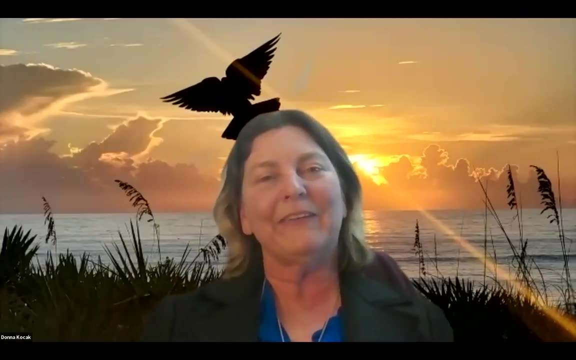 of them. i think you can never mind. i'm sorry, i apologize. well, tell us where's your other master's degree from computer science? uh, ucf, i'm a one-time night or one, a one-time gator and a three-time night- that's a nice combination, all right, i'll disappear for a while, all right, thanks. 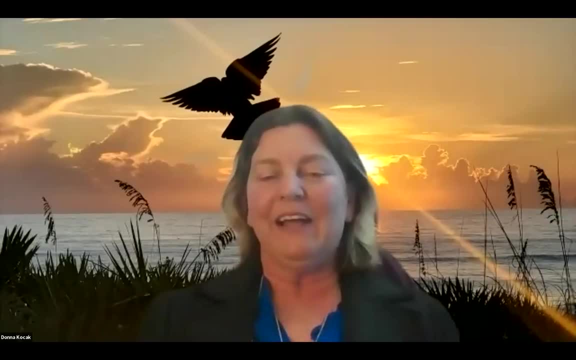 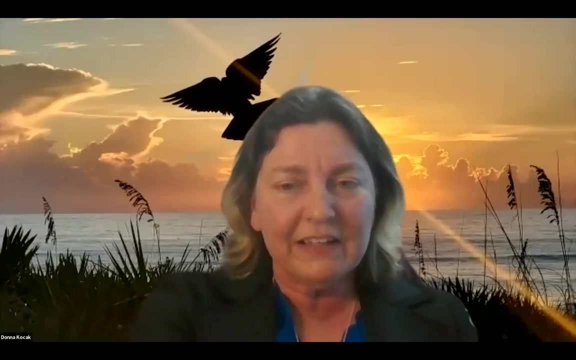 dennis, but i appreciate it. it's an honor for me to be here- uh, virtually you know- giving this presentation where i started my career at uh harbor branch and fau well harbor branch at the time. um, and it's really an honor to talk about this important topic. uh, let me see if i can um bring up my um powerpoint. 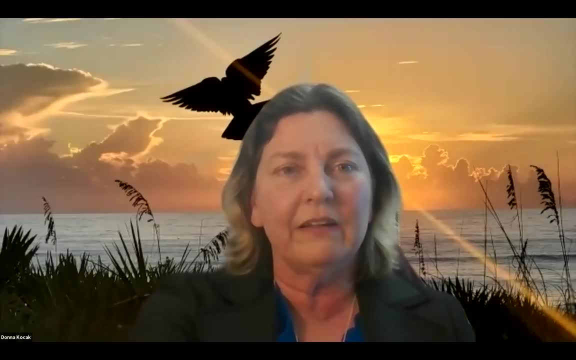 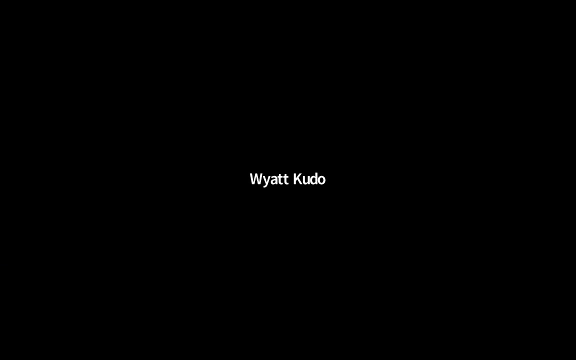 um, now i've forgotten how to do that. um, can you see my powerpoint? i don't think so. yes, you'll want to do a share screen at the bottom and then you'll click the powerpoint. that's right. okay, now i'm not finding the bottom. there we go. 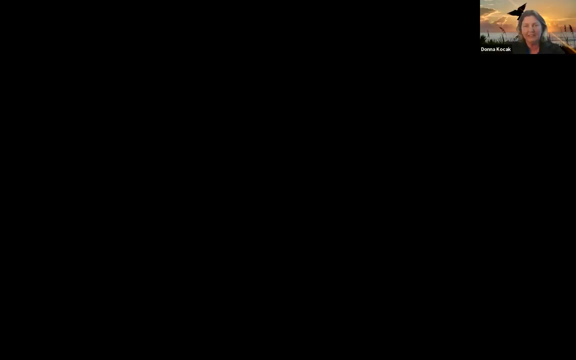 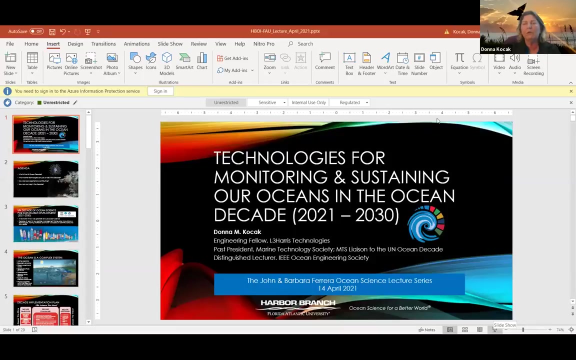 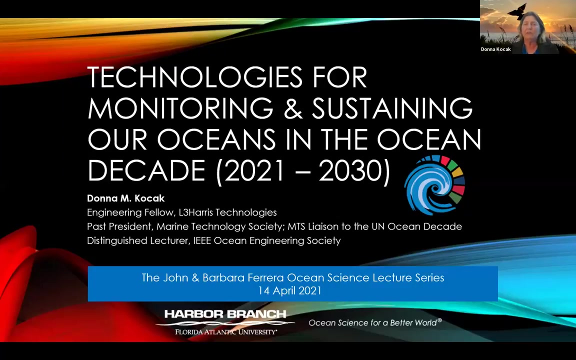 it's a point you have to tell me twice, i guess, okay. so, yes, this is um. get it in powerpoint mode. here we go, everybody can see it, okay. so, um, the topic for today is technologies for monitoring and sustaining our oceans in the ocean decade, that's. 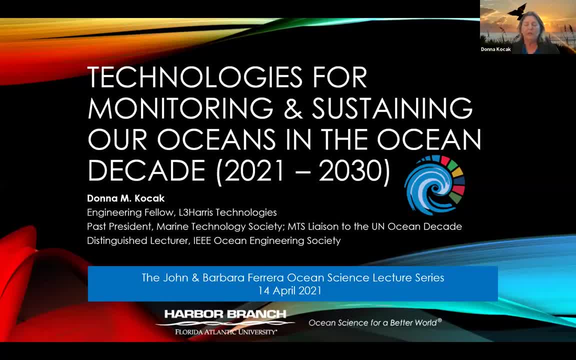 2021 to 2030.. I'm currently, as Dennis mentioned, the marine technology liaison for the decade and I'm excited to share the information about the decade to you. Some of the content in this presentation is recycled from a panel session I participated on in 2019 and Copenhagen. it was the first planning session for the decade. that was really really quite an excitement to be there. 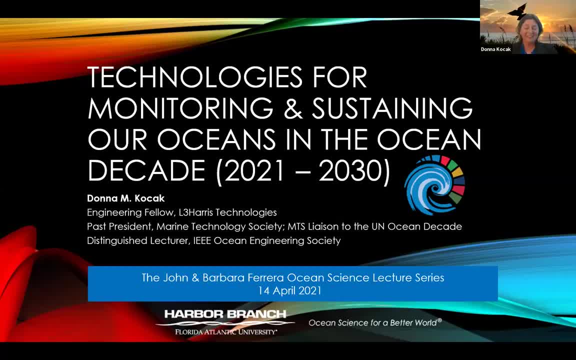 But I'm an engineer by trade, not a marine scientist, So this talk is primarily going to focus on all the awesome new and emerging maritime technologies that can support the upcoming decade. It may not be as interesting as the holy glaciers that's coming up next month, but I hope it will will be exciting to you as it is to me. 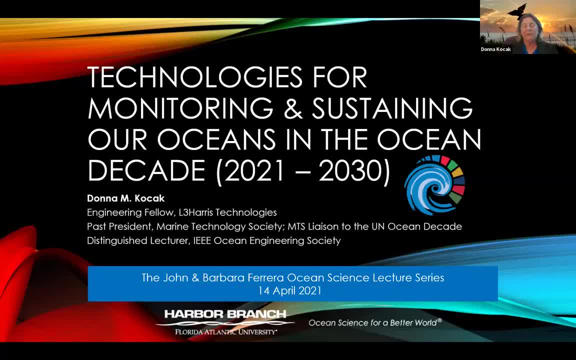 Some of these technologies are going to be presented in more detail in an upcoming special issue Of the Marine Technology Society journal issue in May June timeframe. So if any any of you are MTS members or anything you'll, you'll find more information on this there if you want to join. 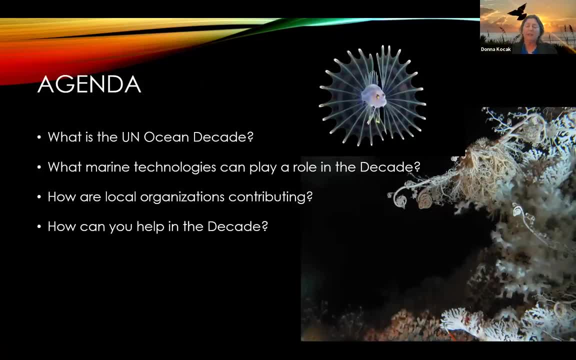 So what I'm going to talk about today, I'll begin with a brief description of the United Nations ocean decade- For short, we can call it the decade- and say why. that's why, why the decade is important to us. I'll discuss some of the innovations. 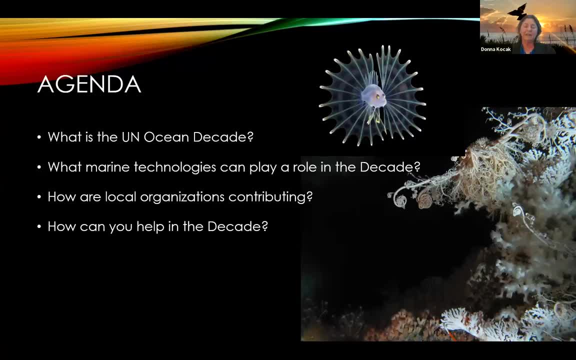 Some of the innovative marine technologies. they can play a role in the decade And some of these examples will be from organizations here in Florida, in our community. so local, local contributions. And then I will provide some pointers on how each of us, no matter where you are, might contribute to the decade. 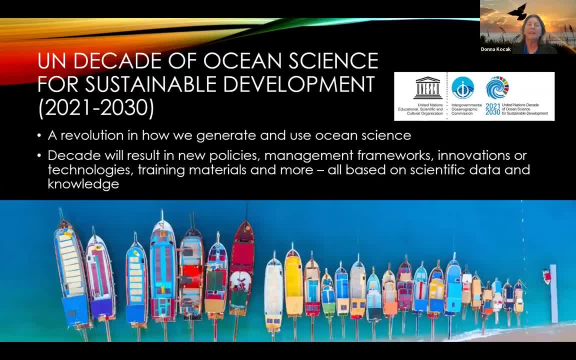 So the United Nation of Ocean Science, United Nations decade of ocean science for sustainable development. What is that? It kicked off in January 2021, 2021, this year, And it was led by the Intergovernmental Oceanographic Commission, which is the IOC of the UNESCO, United Nations, which is United Nations educational, scientific and cultural organization. 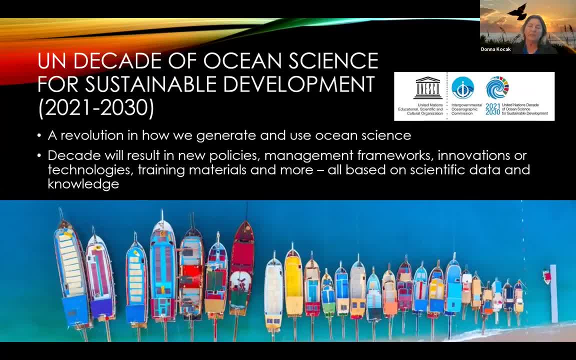 The IOC is a specialized organization of the United Nations system for ocean observations, data services and related capacity development. The decade looks to mobilize the ocean community behind the ideas of sustainable development of our oceans and serves to focus the research and technology, technology development and oceanography on existentially important issues of protection and sustainable use for our oceans. 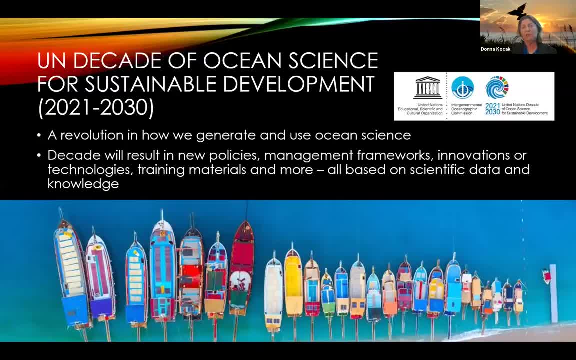 So the decade will also revolutionize how we generate and use ocean science. So the decade will also revolutionize how we generate and use ocean science. So the decade will also revolutionize how we generate and use ocean science and that's that'll be should be very favorable for Harvard branch and FAU scientists. 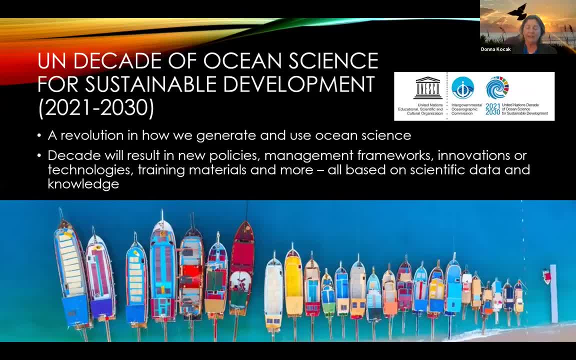 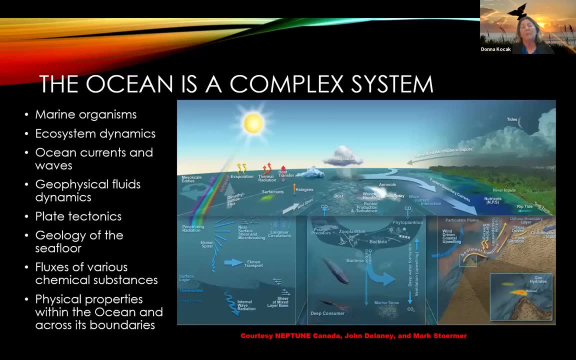 It will result in new policies, management frameworks, innovations or technologies, training materials and more, all based on scientific data and knowledge. So hopefully there'll be more funding and more activities around ocean science so we can improve methods and techniques. So hopefully there'll be more funding and more activities around ocean science. 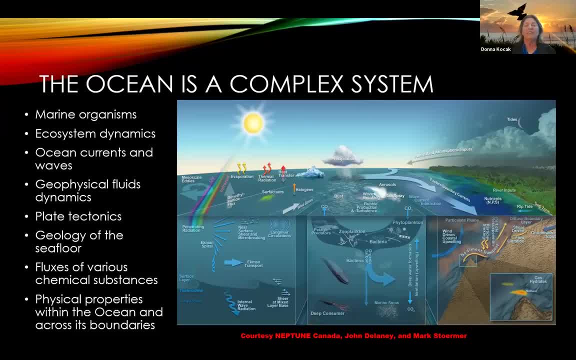 This is one of my favorite photos from Don Delaney- graphic, not photos. graphic graphics from John Delaney at the University of Washington, courtesy of Neptune as well. Canada The ocean is a complex system. you can look at all the things going on in that picture. 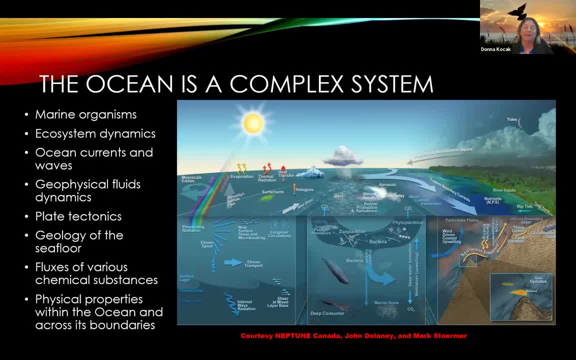 percent of the Earth's surface. It's actually the heart of our planet, providing a range of important services. The seas produce 70 percent of the oxygen we breathe. Deep waters are home to the wildlife and some of the biggest creatures on Earth. It provides us with food, jobs. 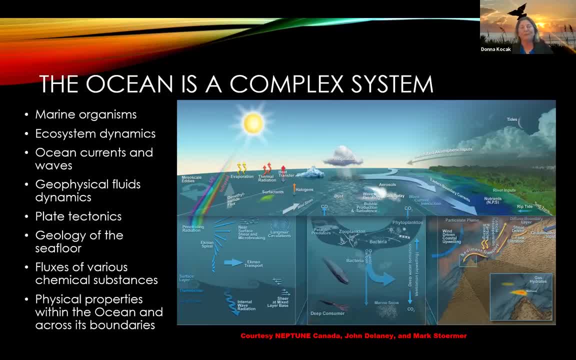 entertainment and diving. As you saw, I'm a diver- Some people might throw in sailing, but a lot of fun things to do on the ocean. To continue to benefit from the ocean, a globally shared information and knowledge system is needed that would inform us actions. 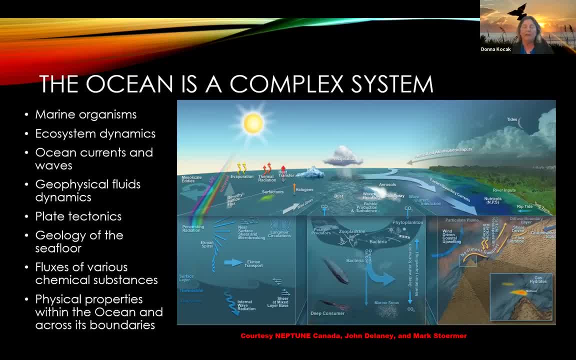 for the restoration and maintenance of the ocean's health, and use of the ocean's space and resources to achieve global sustainable development. Data collected on the global environment will help us better understand this complex picture that we're looking at. This will involve marine organisms, ecosystem dynamics. 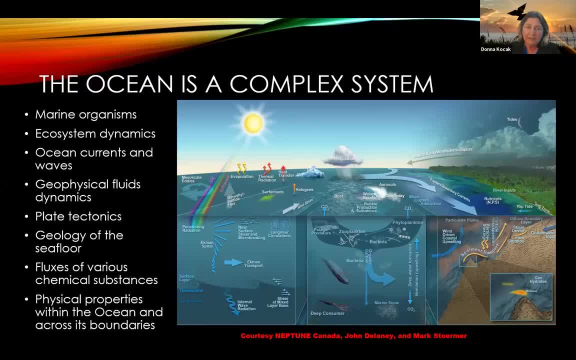 oceanic and marine life and the development of marine life, Ocean currents and waves, geophysical fluid dynamics, plate tectonics, geology of the sea floor, fluxes of various chemical substances and physical properties within the oceans and across its boundaries. So there's a large amount of science to be learned here. 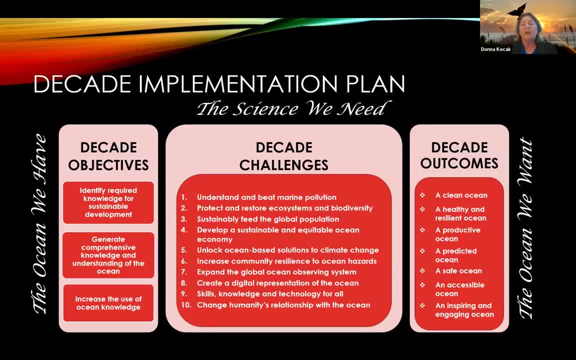 The decade has an implementation plan and it also has a slogan. The slogan is: the ocean we have, the science we need, and then for the ocean that we want. So they've outlined that. IOC has outlined a number of decade objectives, the challenges to those objectives. 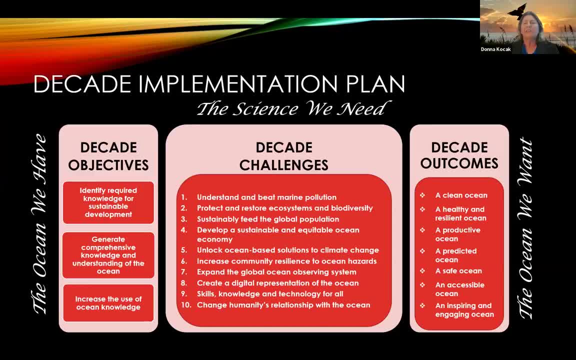 and then the outcomes that we hope to accomplish through these 10 years. The objectives, if we're looking over here on the left-hand side, in the first box, identify required knowledge, underpinning infrastructure and partnerships for sustainable development. It'll be important to establish partnerships in this. 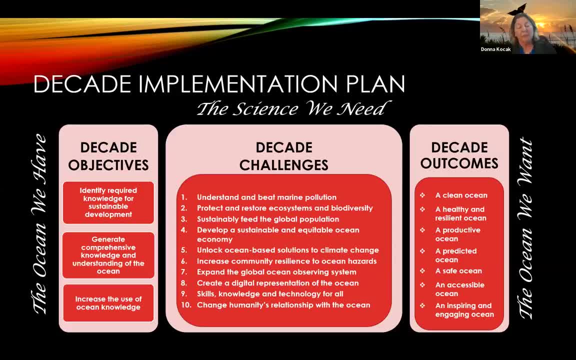 large global effort Generate comprehensive knowledge and understanding of the ocean, and we'll do that by collecting data. and better understanding that picture that we just looked at Increase the use of ocean knowledge. So once we get this knowledge, let's go ahead and use it. 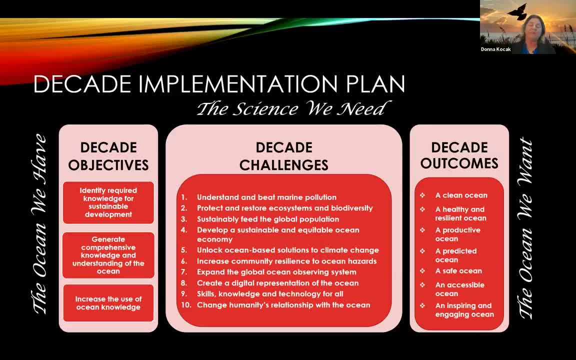 One way to use the ocean science is for data to inform policy making. So the challenges? I've listed 10 challenges. First is understand and beat marine pollution. I don't have to tell you about the changes that are happening in our oceans. Most people are aware of the Great Pacific Garbage Patch. 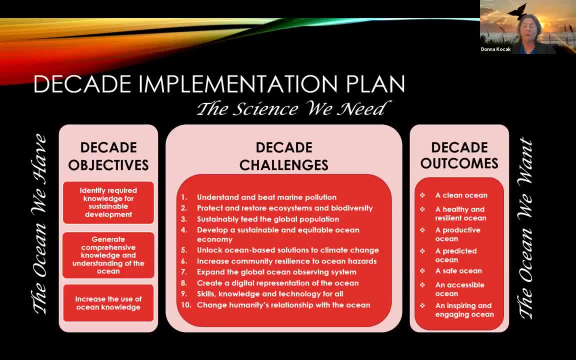 This is part of the five offshore accumulation zones of plastic in the world, and this one is located halfway between beautiful Hawaii and California. It's approximately twice the size of Texas. It's one of the largest in the world And it's located halfway between beautiful Hawaii and California. It's approximately twice the size of Texas. It's one. 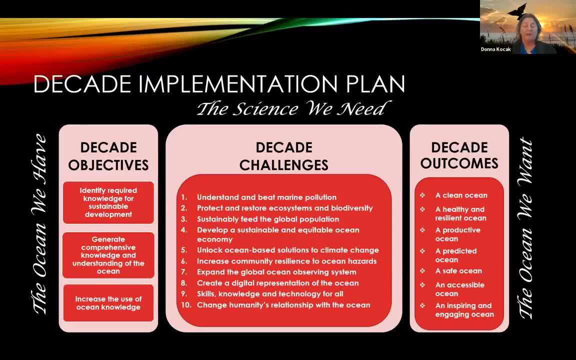 point, six million square kilometers. So the next challenge is protect and restore ecosystems and biodiversity. We're currently experiencing an escalating loss of marine life. We should we need to stop that- Sustainably feed and feed the global population. So over three billion people rely on fish for a substantial part of their protein. 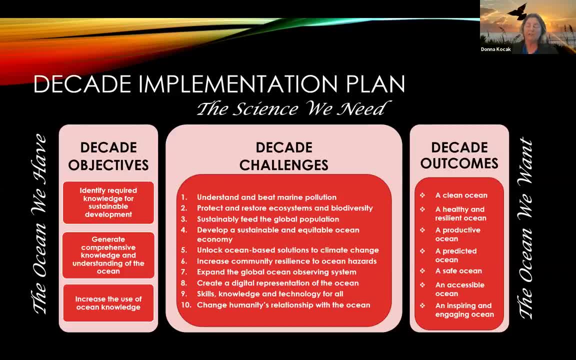 Develop a sustainable and equitable ocean economy. This can include shipping, tourism, offshore energy and other areas that are probably still yet to be defined. Unlock ocean-based solutions to climate change. Use and use these these solutions to get better predictions for the ocean. 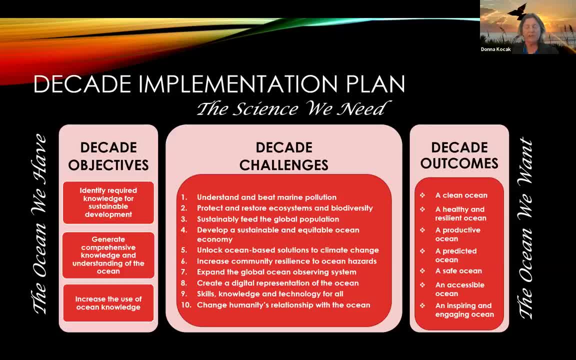 climate and weather. Increase community resilience to ocean hazards. This can include early warning systems for tsunamis, hurricane protection, rising sea level and other impacts to ocean hazards. Expand the global ocean observing system by delivering accessible, timely and actionable data to all of its users. Create a digital representation of the ocean. 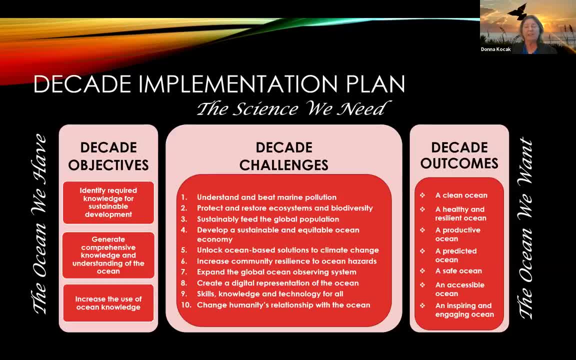 such as a dynamic ocean model that has free and open access for exploring, discovering and visualizing past, current and future ocean conditions, And we want to make this available to all of the stakeholders. Skills, knowledge and technology, me, 저 and technology for all, including capacity development and equitable access to data. 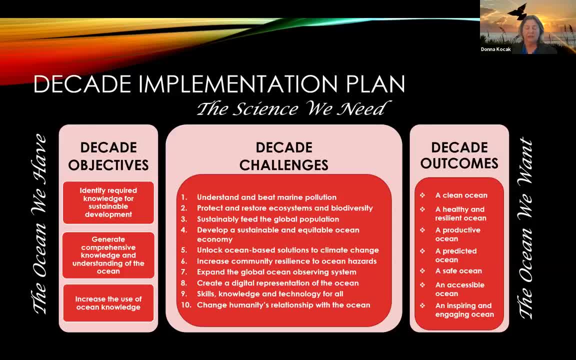 information, knowledge and technology And change humanity's relationship with the ocean. Human well-being, culture, sustainable development are widely understood, but we may need to identify and overcome barriers to behavior change. So all of these should, we hope, boil down to the decade outcomes, And I list seven decade outcomes. 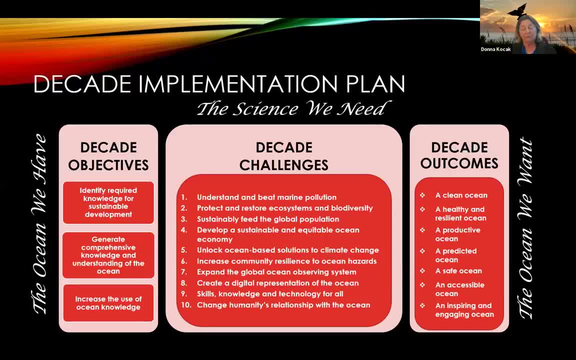 here that are very important in the next 10 years. The first is a clean ocean, where sources of pollution are identified and renewed. A healthy and resilient ocean where marine ecosystems are mapped and protected. A predictable ocean, where society has the capacity to. 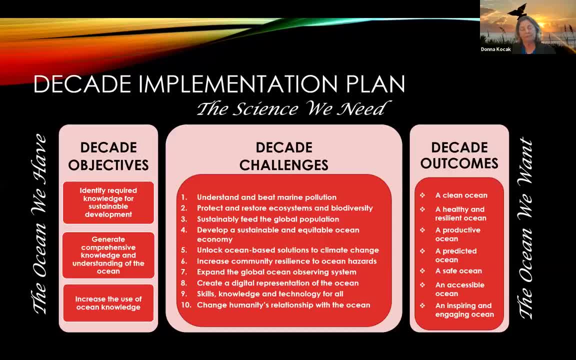 understand current and future ocean conditions. A safe ocean, where people are protected from the ocean hazards. A substantially sustainably harvested ocean, ensuring the provision of the food supply. A transparent ocean with open access to data, information and technologies. 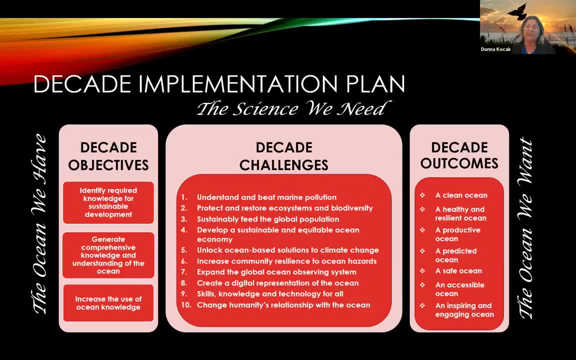 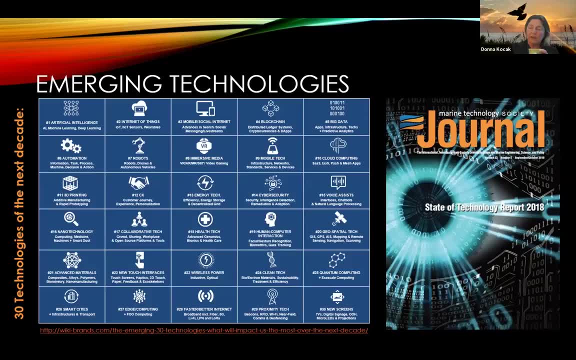 And an inspiring and engaging ocean where society understands the value of the ocean. So that's my science portion of the talk. I'll get into the fun part here. This is the emerging technology portion. This is the graphic. here is somewhat of an eye chart. 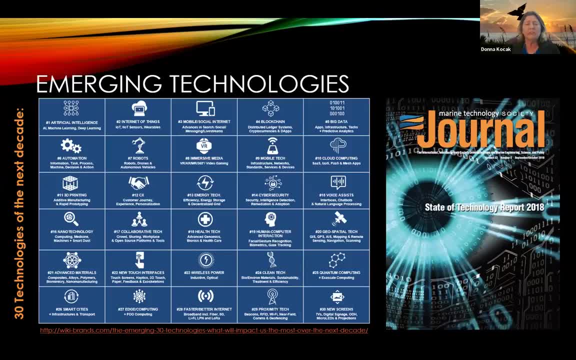 but it's actually one of my favorites. The table shows the next uh, the top 30 technologies of the next decade, And this was published in 2018, so it's a couple years old. I included this in the last section here and I think that it's in the next slide. And so this the next slide, and this was published in 2018, so it's a couple years old. I included this in the last section here and I think that it's an interesting one. So even a small portion of the talk. 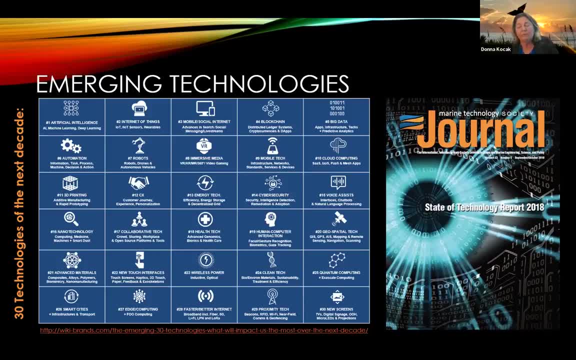 this in a special issue of the Marine Technology Society's journal of the 2018 State of Technology Report on the right. I won't read all of these top three, but I will highlight a few And I'm going to relate the next emerging technology back to this chart. So artificial intelligence is. 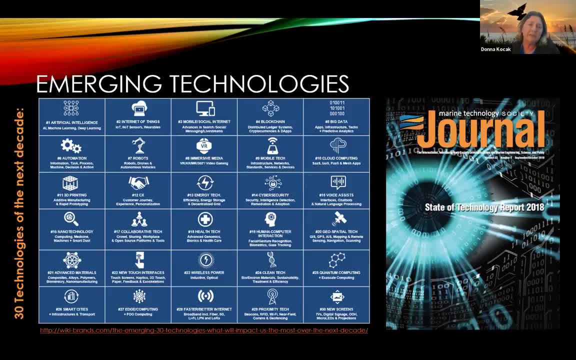 perhaps the number one technology of the decade. This includes AI, machine learning and deep learning. The second one is pretty big too. It's the Internet of Things. So it's the Internet of Things, sensors and wearable sensors, and just the Internet in general. Number five is big data. 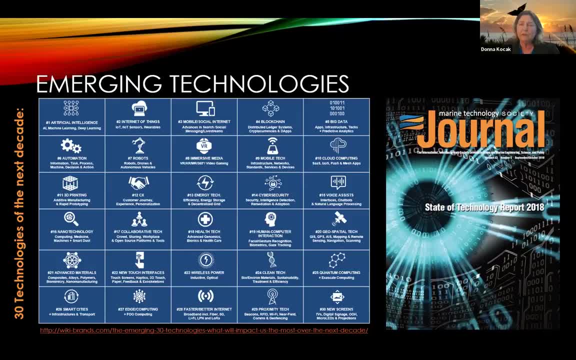 That's one that comes up a lot. It includes apps, infrastructure technologies and predictive analytics, And I like number seven. I'll be talking about that a couple times. Number seven is robots, So there's robots, Drones and autonomous vehicles, So we'll carry on here. There is a link here, So if you go back, 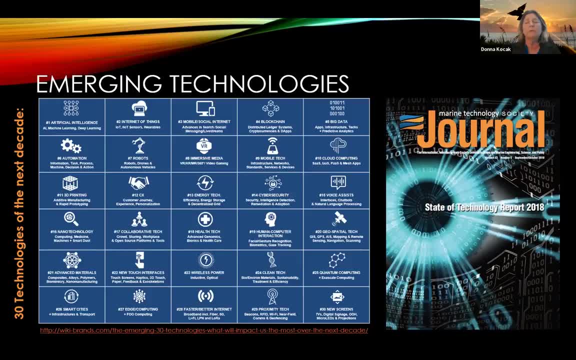 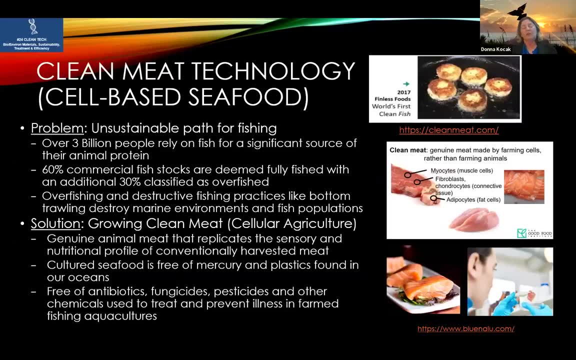 and want to reference this chart. it should be at the link accessible, Or if you have the MTS journal, you'll find it there. So the first one I'm going to talk about. the first technology relates to the clean technology. It was number 24.. This is something you may or may not have heard. 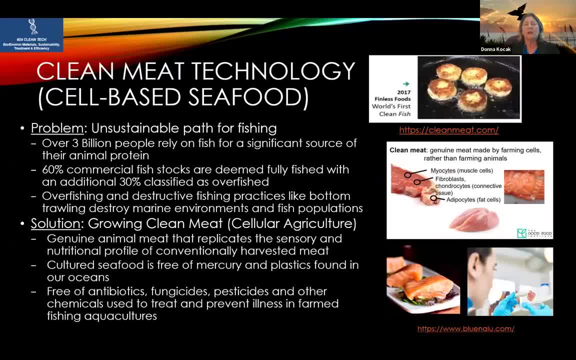 of You've heard a lot about aquaculture. I'm sure you've heard a lot about plant-based food, But this is something different. This is clean meat technology. It's also referred to as cell-based seafood or cellular agriculture, And I'm not sure if growing meat in a petri just sounds appetizing. 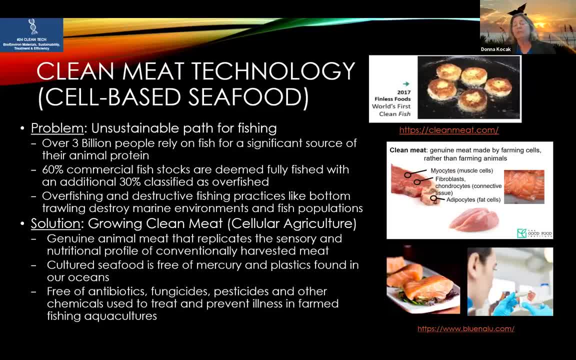 or not, But I think it's very important for the future of the world. The problem is we have an unsustainable path for fishing. Over 3 billion people, as I mentioned earlier, rely on fish for a significant source of their animal protein And 60% of the commercial fish. 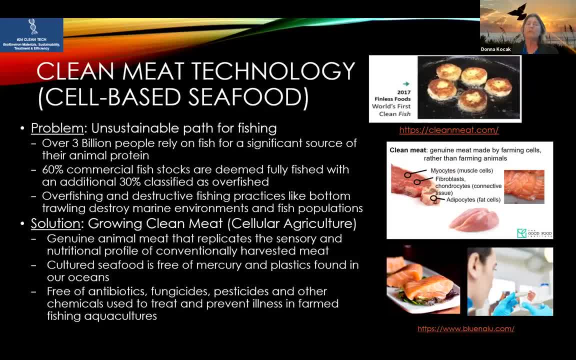 stocks are deemed fully fished, with an additional 30% classified as overfished. Overfishing and destructive fishing practices like bottom trawling destroy the marine environments and the fish populations. So the solution we have here is a growing clean. 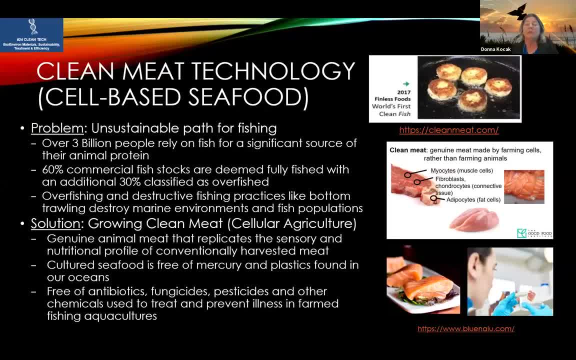 clean meat. I also like to say 3D printing. So basically you take an actual cell from a salmon, a tuna, whatever fish it happens to be- And this can work for meat as well- And you grow that cell. So if you want the certain prime part of the salmon that you have in sushi, 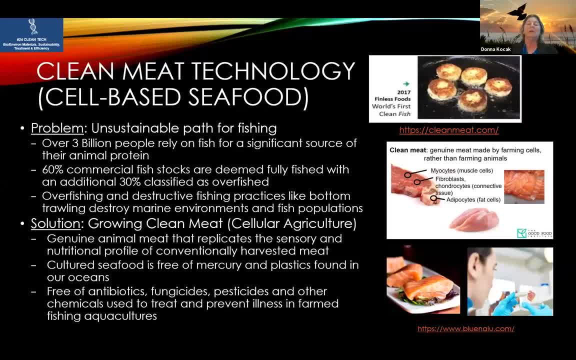 in that picture down there you can grow just that portion, So it requires a cell once And then you don't use any more. It's genuine animal meat that replicates the sensory and nutritional profile of conventionally harvested meat, So it tastes just like real meat. It looks just like real meat. 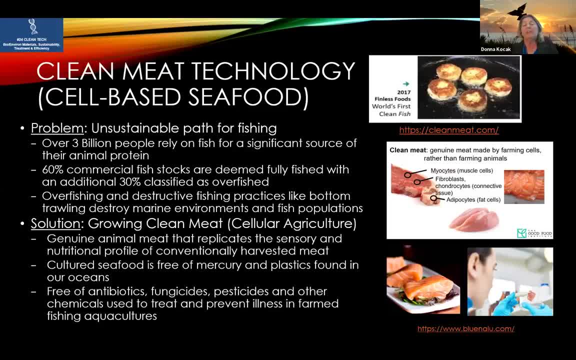 And the preparation and all is just the cooking of it. It's like real meat, Cultured seafood. This is cultured. It's free of mercury and plastics that are found in our oceans. As we're finding out, there's a lot of things in our food that we probably don't. 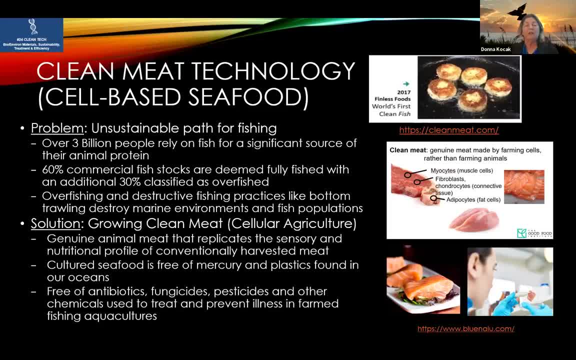 know about. So it's free of mercury and plastics that are found in our oceans. As we're finding out, there's a lot of things in our food that we probably don't know about, about the plastics, and even in our body Culture. so it's free of antibiotics, fungicides, pesticides. 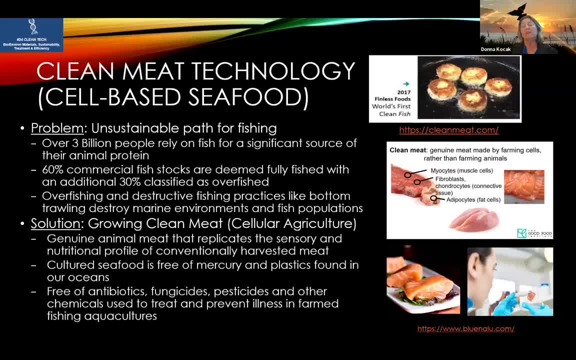 and other chemicals that can be used to treat and prevent illnesses in fishing. aquaculture fish farming- Not that fish farming is bad. there are a lot of ways to farm fish. One company, Finless Foods, shown in the upper right-hand corner, actually grew the first. 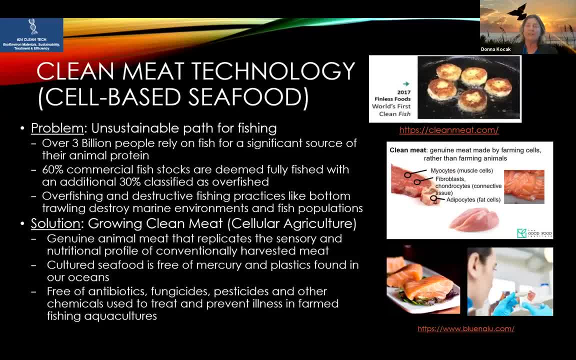 finless clean fish in 2017.. And there's another company, Blue Nalu, in San Diego, that recently demonstrated its yellowtail product, showing that it could be prepared in the raw form, the cooked form: it was seared, grilled, broiled fresh, fried and microwaved and prepared via acidification. So 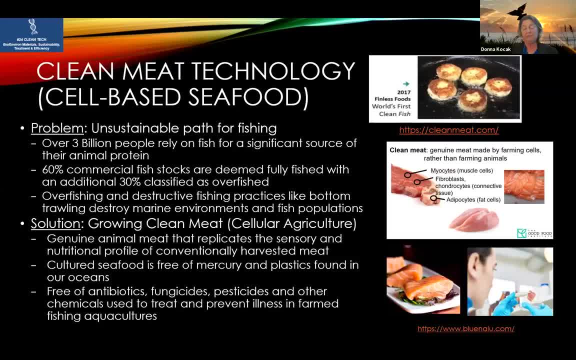 in ceviche, poke and kimchi foods, But that doesn't make me hungry. now it's almost dinner time, So keep an eye out for that. Keep an eye out in the grocery store in the near future for these types of products. Right now, 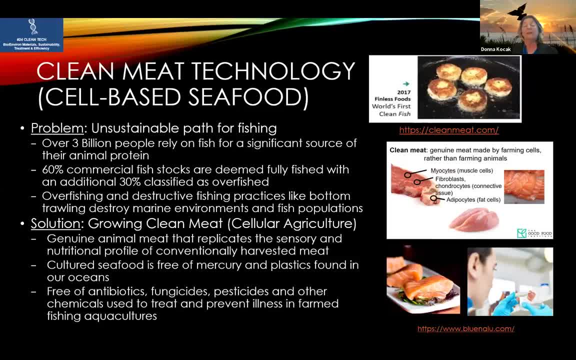 they're still pretty experimental, so they're really expensive. But as we start to make this more, get this more to the mainstream, the price will go down And then we can live with our buddies in the ocean and catch fewer of them. 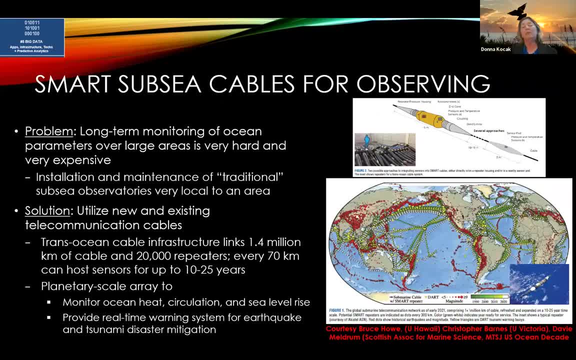 The next one I want to talk about is a smart subsea cables for observing- And I threw this in the chat, but it's a really good one. It's called the Smart Subsea Cables for Observing, And I threw this in the chat, but it's a really good one. It's a really good one. It's called the Smart Subsea Cables for Observing. 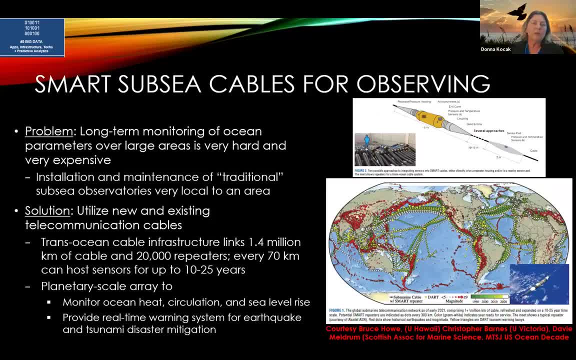 And I threw this one into the number five big data category because of the infrastructure which would cover the telecommunication cables on the seafloor. So in order to get the data, we need to learn more about science and our planet. it requires long-term monitoring of the ocean parameters over large areas in the ocean. 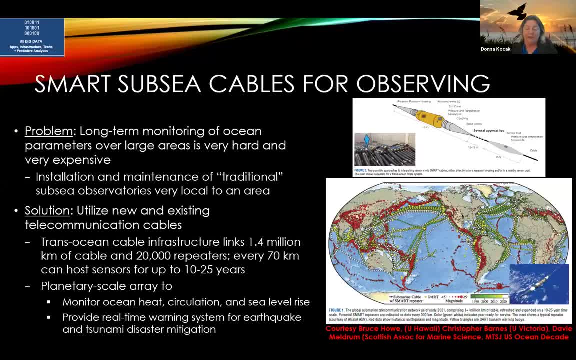 And that's very hard to do and very expensive. And that's very hard to do and very expensive. There's a lot of individual data that I've gathered over the last few years- individual installations, ocean observatories around the world- but they occupy a small area. 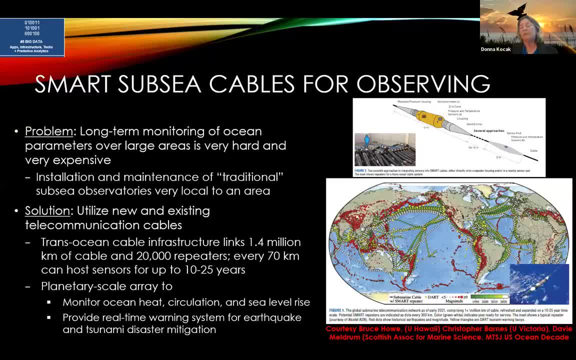 not the whole ocean: Neptune, Canada and the regional scale nodes in the Pacific Northwest. offshore There's the Mars Observatory in Monterey Bay Donut in Japan, mainly used for tsunami early warning, but just local in Japan. The offshore communications backbone in Cyprus. 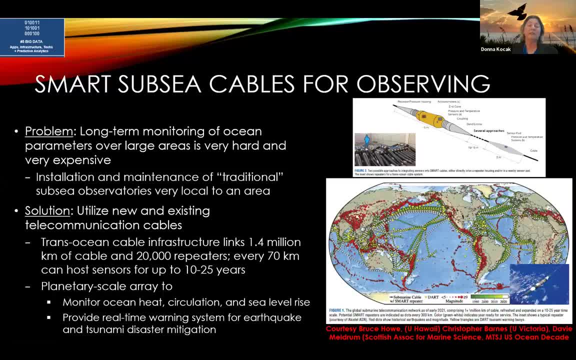 for monitoring oceanographic data and tsunamis. So there's not an easy way to gather data all across the globe and our oceans. The solution we're proposing here- this is actually being proposed by University of Hawaii, University of Victoria and a Scottish Association for Marine. 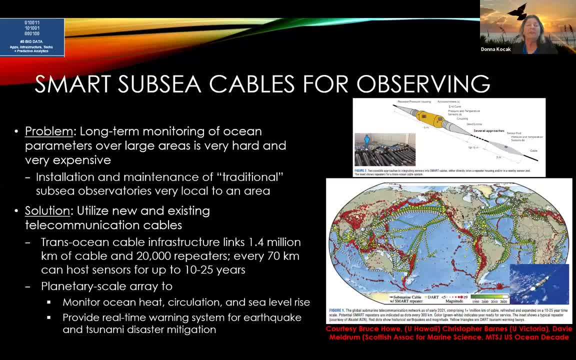 Science Collaboration And it'll utilize new and existing telecommunication cables. So Transocean cable infrastructure links 1.4 million kilometers of cable and 20,000 repeaters, And I show the picture of a repeater up there. The repeater just allows an optical communication. 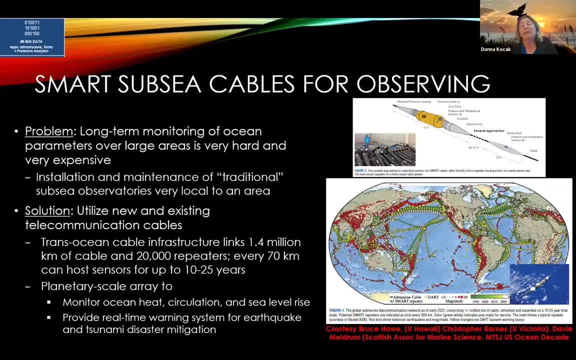 signal to be regenerated and transmitted further. So typically your optical signal can go 120 or so kilometers and then there's enough loss to overcome that signal that you need to regenerate it to send it out again. So that's a lot of repeaters. 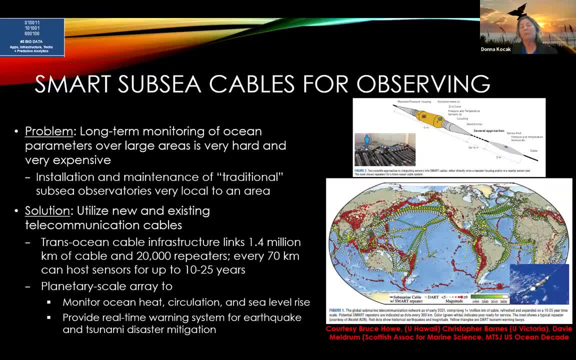 And every 70 kilometers or so they typically deploy the repeaters or 85. And it can host a number of sensors inside of that repeater for up to 10 to 25 years. Typically subsea telecommunication equipment is 25-year life, So think about putting sensors inside of the repeaters and having them. 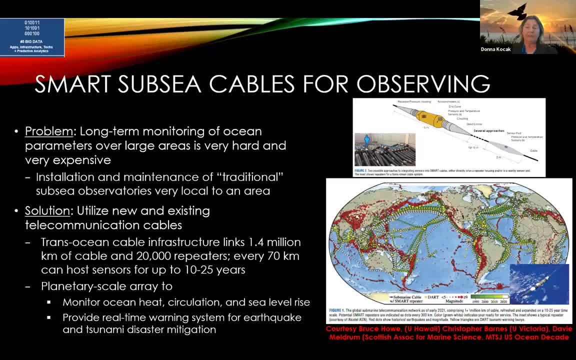 accessible all around the world on all that fiber that's already down there shown in the picture. So that's a high-speed internet connection, So it's a planetary scale array, And what they want to do is monitor ocean heat circulation and sea level rise with pretty simple sensors and eventually, 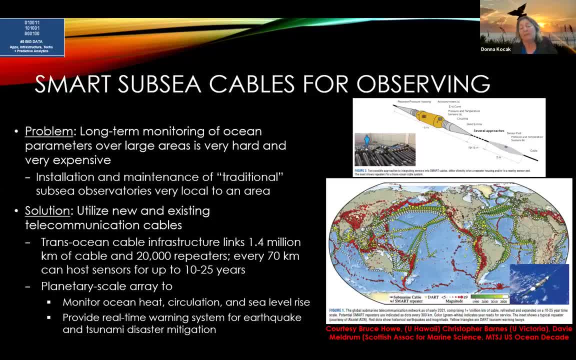 provide real-time warning system for earthquake and tsunami disaster mitigation. So we'll be able to detect a wave, tsunami wave- as it crosses the ocean, with enough time to provide an early warning. So that's a novel, a novel technology. We'll be presenting this in the NTS journal issue coming up on the ocean decade. There'll 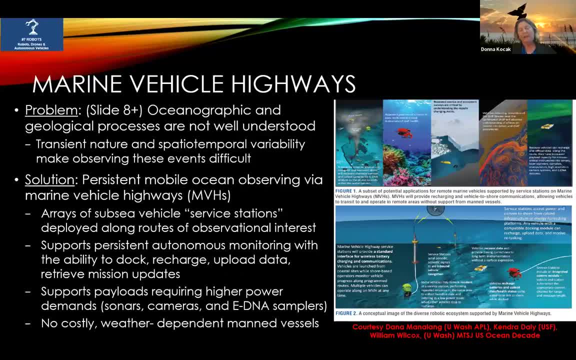 be more details there. The next technology is pretty novel as well. It's being proposed by the University of Washington, APL Applied Physics Lab, University of South Florida, and the University of Washington in general. This is Marine Vehicle Highways, So it's. 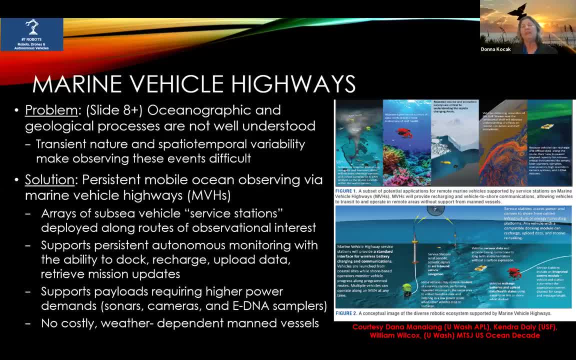 a similar concept as the last one, trying to gather data from across the oceans, But it's targeted more towards the long-term geological processes where transient nature and spatial temporal variability make ocean observing events difficult, And this can be tectonic plate shifts, with the chances you're going to catch that event, or seafloor spreading. 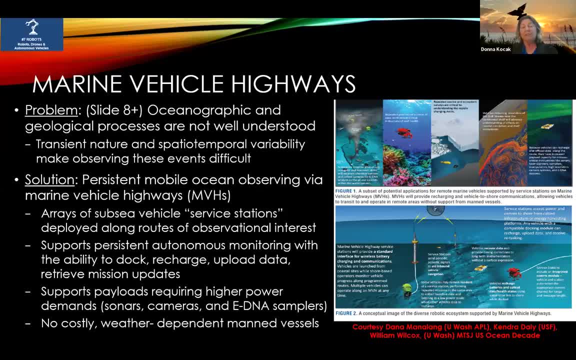 that can cause a submarine volcanic eruption, the avalanches or the earthquakes. So it's trying to catch those events that are that are difficult to capture, And to do this a lot of the technologies are being being developed in the research and DOD community. So bringing this, bringing this into one piece, is not a long, it's not a. 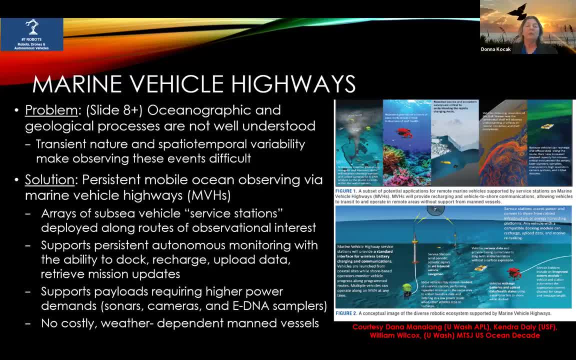 long shot it's not unfeasible. So it would consist of arrays of subsea vehicles' service stations, So it's like putting down a recharging docks and rating engine for each one of these lumethrou, directly traveling into the novels who perform tasks and results, and it's an online. factories breath in reading And so it's hard. so the industry can and is transported freely. it would be shameless. So it's designed in terms of- maybe you know, doing complete research to engage all these male celebrities who are, you know, into a Forward Option or supporting the 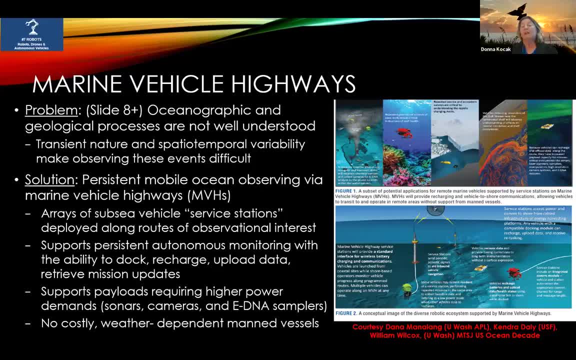 surveys and how it may be count today. And we've also been able to discover the recharging docking station, So an underwater vehicle can pull up onto it and be serviced. It could be recharging, there could be data downloading and also mission uploading, So it 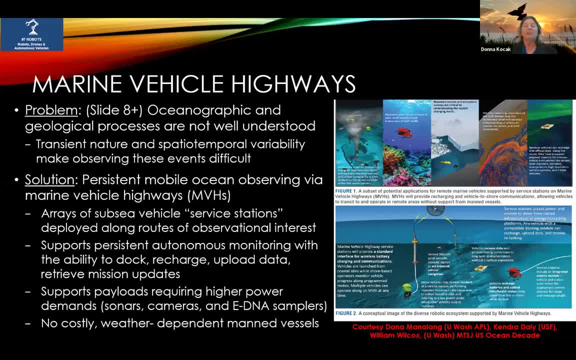 can actually connect to the internet to provide that two-way communication, And these would be put, these service stations would be put along routes of interest. So John Delaney at the University of Washington was interested in the Juan de Fuca Ridge and the tectonic plates and 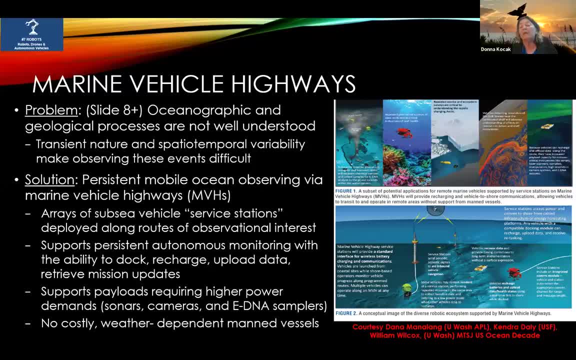 the underwater volcanoes. So putting them in that area, around the plates of the volcanoes, would be a likely point. Putting them near hydrothermal vents: if you're collecting energy from hydrothermal vents, that could be another way harvesting the energy of the ocean. 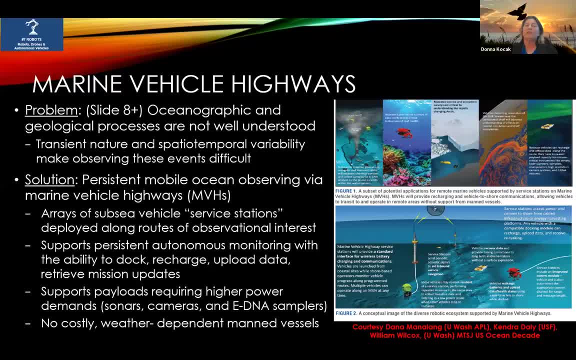 So this supports persistent autonomous monitoring with the ability to monitor the water quality of the ocean. So this supports persistent autonomous monitoring with the ability to monitor the water quality of the ocean. So this supports persistent autonomous monitoring with the ability to dock, recharge, upload data and retrieve mission updates. 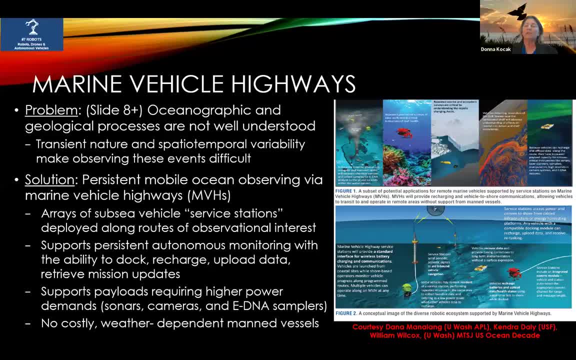 It supports payloads requiring higher power demands. So because you're there with power available, you can run sonars, cameras and eDNA samplers that require a large amount of power. The lights and the cameras typically require high voltage. And because you're down there, 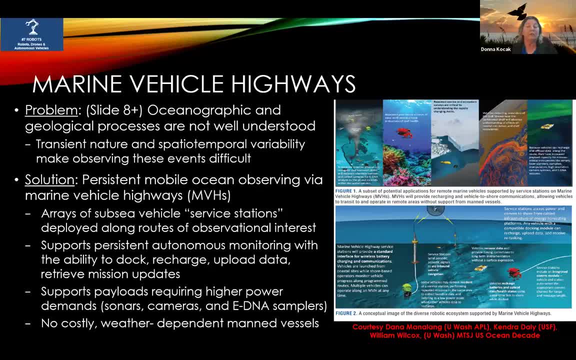 persistently and it's an infrastructure that's there for a long time duration. there's no costly, weather-dependent man vessels. You don't have to go out there to service it, maybe periodically if there's a failure or preventative maintenance, but you don't have to sit there with a ship. 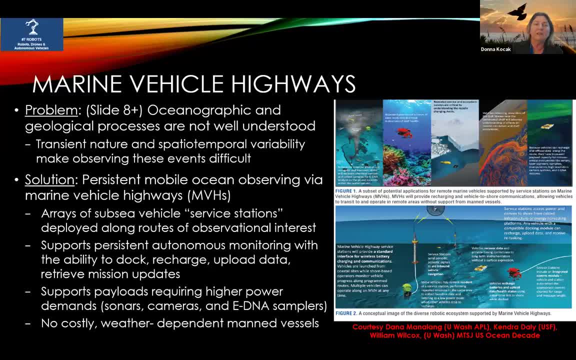 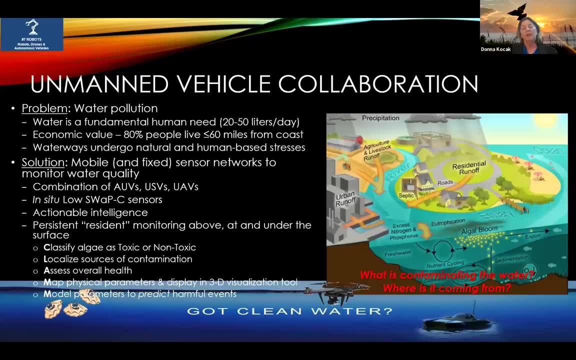 And this one was my first robotic category one with the robotic drones. So we have drones and autonomous vehicles. The next one that's also in the robotic category is the unmanned vehicle collaboration. So this is a robotic vehicle collaboration. So this is a robotic vehicle. 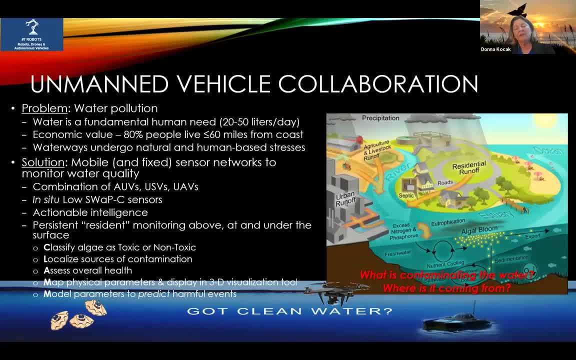 collaboration. So when I say unmanned vehicles in the maritime field, there's the unmanned surface vehicles, USVs, there's the unmanned underwater vehicles, which are the UUVs, and then sometimes these can cooperate with the unmanned aerial vehicles, which are the UAVs. So down the bottom. 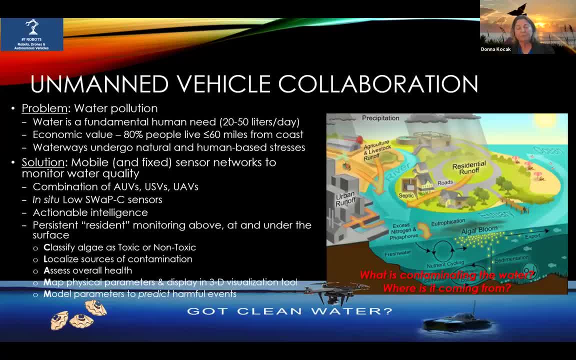 there I show a surface vehicle and a UAV. The trend for these vehicles is not only to team with human the human counterparts- where you'd have to team with the human counterparts but you'd have the human machine teaming- but also to team with each other. So we have the machine to machine. 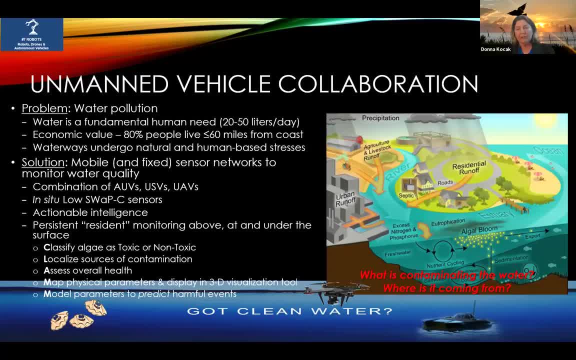 teaming. And if we look, you know what is the problem that we're addressing with this vehicle collaboration. So it's water pollution. So water is a fundamental need for humans. And what's splintered out too is 80% of the people live 60 miles or less from the coast. So if we look at 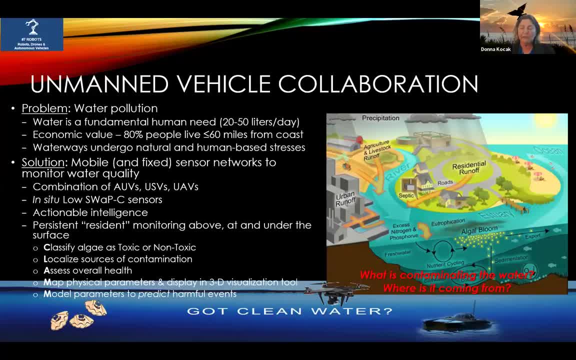 the picture, there's a lot of water pollution. So if we look at the picture, there's a lot of runoff there. The health of the oceans and waterways are impacted by multiple natural and human-based stresses. Everything from land is an influence and every drop of rain is an influence. 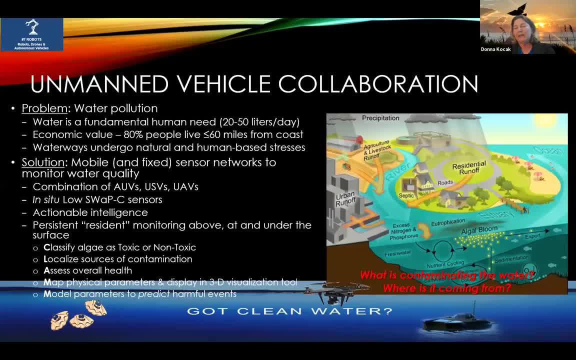 to the water. So what is contaminated in the water and where is it coming from are two important concerns. We've seen in Florida, along the East Coast and West Coast. we've seen the tragic effects of red algae blooms. We've seen, you know, we've seen, you know, we've seen, you know. 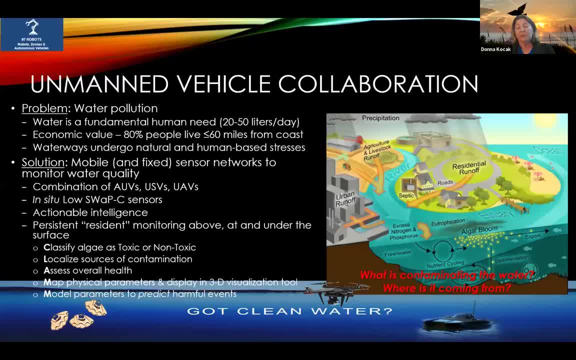 and fish kills. So these are some of the things we want to try to help prevent. It's critical to monitor and understand the variations in the state of the health in order to localize the root causes and mitigate their effects, just as a doctor would monitor their patients in intensive care. 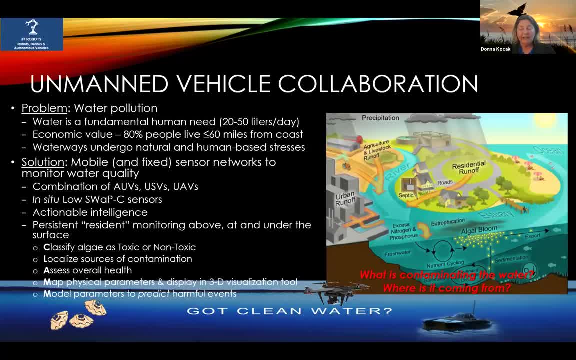 Locating sensors in fixed locations and having a mobile network that can help gather the data is what we're proposing here. So, in particular, we want to find a way to track down the sources of contamination, which is vital for restoring and mitigating further degradations. So, as I said, we're combining multiple types of 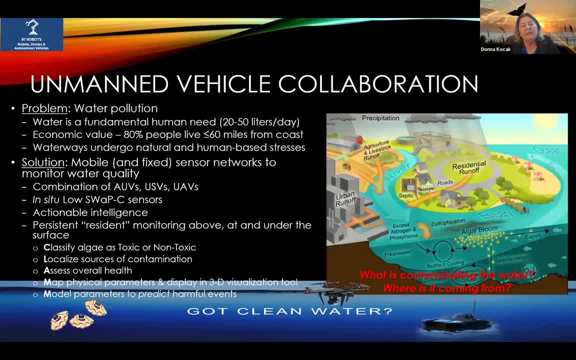 sensors- AUVs, USBs and UUVs actually- And then we would be putting low swap, which is size, weight and power, and a dash C is the cost. So low cost, low size, low weight, low power sensors on these. 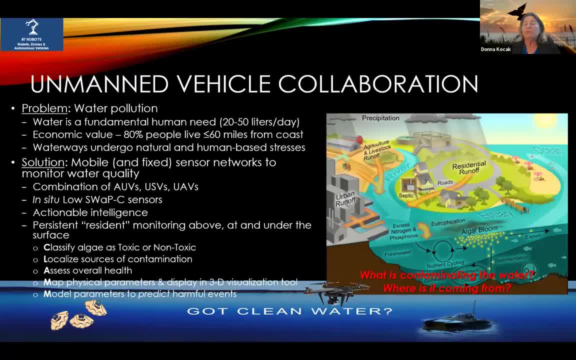 vehicles. They would be out there collecting actionable intelligence, meaning if one of your fixed sensors or one of your mobile sensors discovers a contaminant, real time it could take action. It could try to follow the track of the contamination up the river and see where. 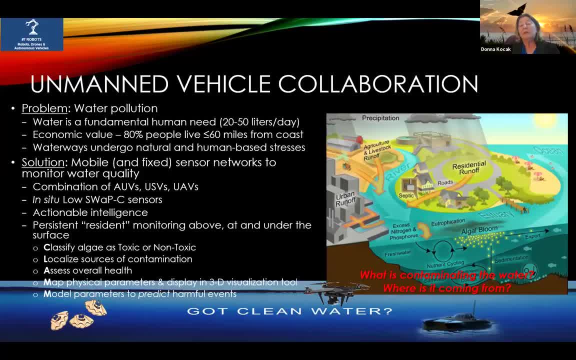 that's coming from? Is it coming from a septic tank area? Is it coming from cows in a pasture agriculture type flow from land? Or did a gate just open up, a water control gate, And something came down the river to contaminate? So there's a chance of trying to find it, But what? 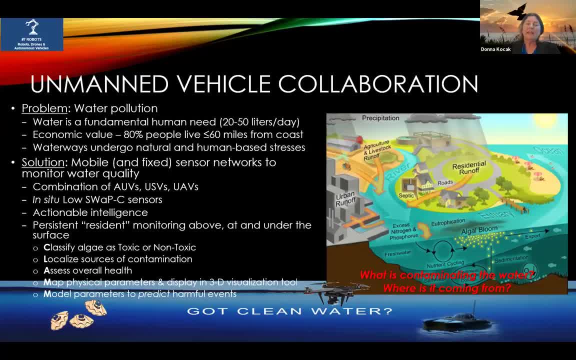 you would do is have the vehicles remain persistent and resident above water, at the water surface and then under the water, And I have a little acronym here. One of our ideas was to classify algae as a toxic or non-toxic as clams, Localize the sources of contamination, assess the overall health. 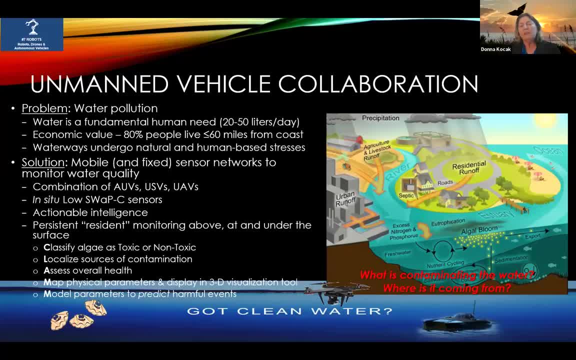 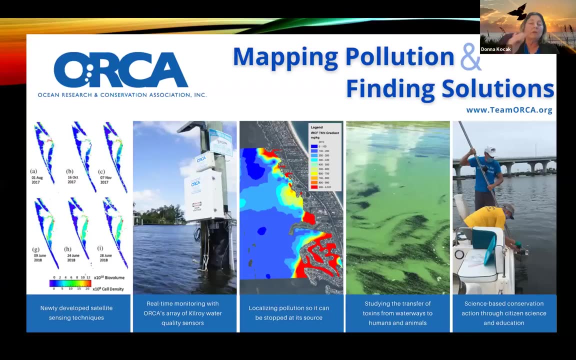 map physical parameters and display in a 3D visualization tool and then model the parameters to predict the harmful events. So the whole goal is to collect the data to be able to monitor back and prevent further events and to help clean up the oceans. There are, there are several, there are at least two. 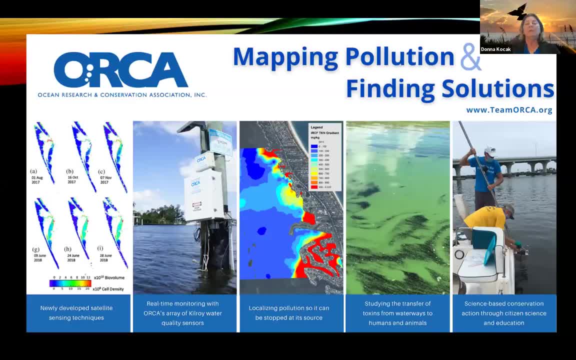 that I'm going to talk about sensors that exist and they're the fixed sensors right now. But Orca is a great example here of sensors on the water, and they're the fixed sensors right now. but Orca is a great example here of sensors on the water. 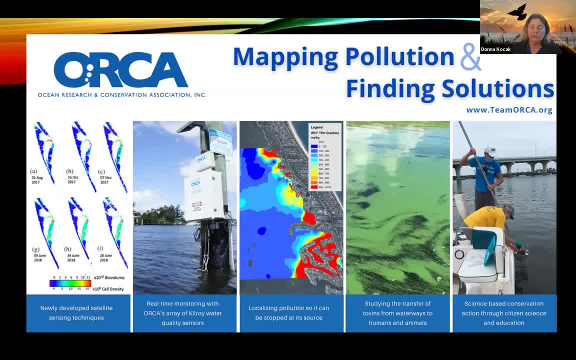 the Indian River Lagoon. ORCA is the Ocean Research and Conservation Association. It's headed up by Dr Edie Witter. She's a former Harbor Branch scientist and she was my computer vision master's committee advisor- one of them- So I looked at her bioluminescent critters. 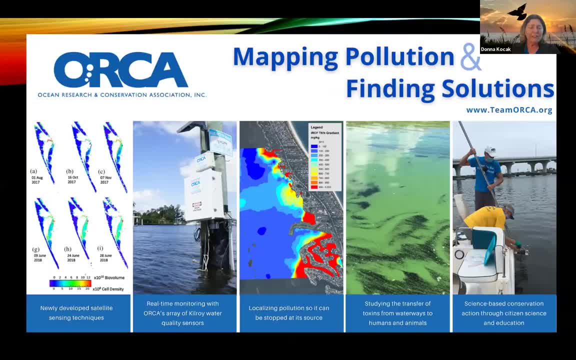 for my master's degree, And on the left-hand side you'll see newly developed satellite sensing techniques. So Edie combines satellite data here, remote sensing a brown tide bloom using a satellite and ground-based hyperspectral spectroradiometers, in collaboration with 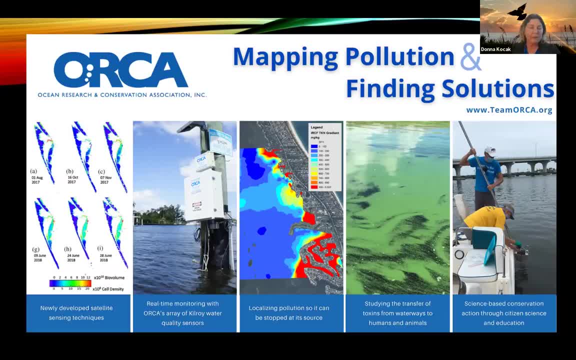 Kent State University. So the map here shows the time series from August 1st 2017 to November 21st 2018, of 12 spatially distributed maps, A through L, which correlate positively to the brown tide signature. There was a published article on this In all of the 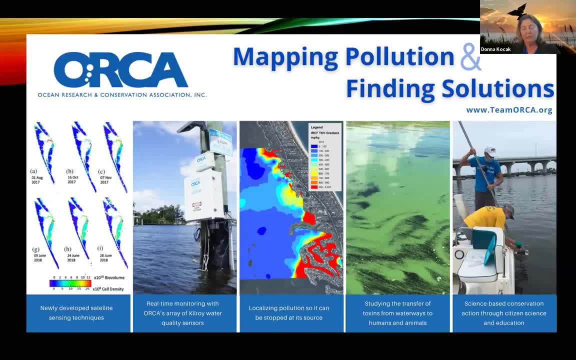 images. the warm colors indicate higher biovolume or cell density, the cells per meter- while the cool colors indicate lower powers, lower values. The next panel here, from the left to the right, is real-time monitoring with the ORCA array of Kilroy water quality sensors. So it's showing: 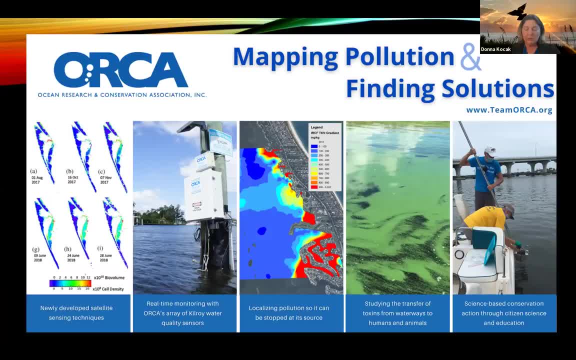 a Kilroy sensor deployed in the Orca And it's showing a Kilroy sensor deployed in the Orca, And that's what we're talking about here at the Indian River Lagoon, providing real-time monitoring data which is available at wwwTeamORCAorg. So there's currently 18 of the Kilroy in the 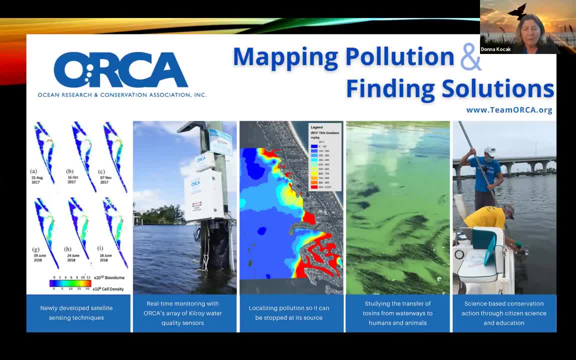 Indian River Lagoon. Panel three is localizing pollution so it can be stopped at its source And, as I mentioned, that's a very valuable thing to do. That's the goal of getting rid of the contamination. So pollution mapping of nutrients and toxins in sediments. 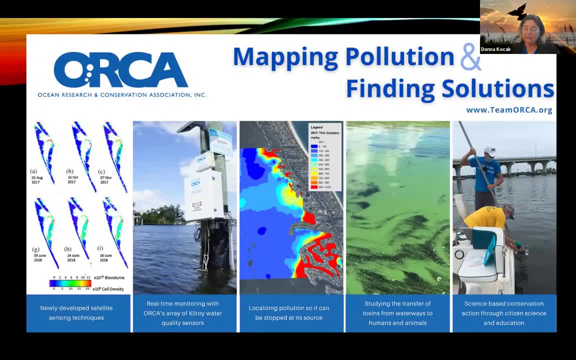 there's clear evidence of the critical importance of living shorelines has led to the major emphasis on restoring living shorelines, So it would impact a lot of the beach erosion and land bringing in sand that we're working with here. Panel four is studying the transfer of toxins. 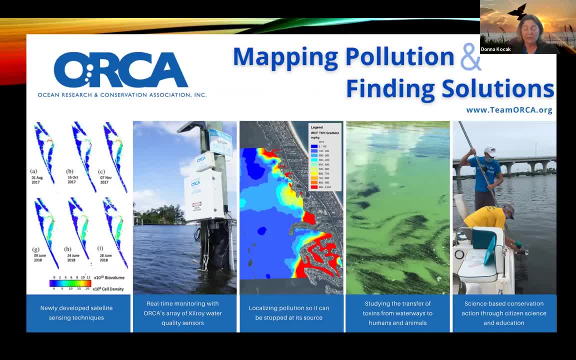 from waterways to humans and animals. That's an interesting concept, where ORCA's One Health program focuses on studying how toxins from toxic algae blooms and toxicants such as herbicides and pesticides are making their way into humans and animals. And finally, on the right is ORCA's new Center. 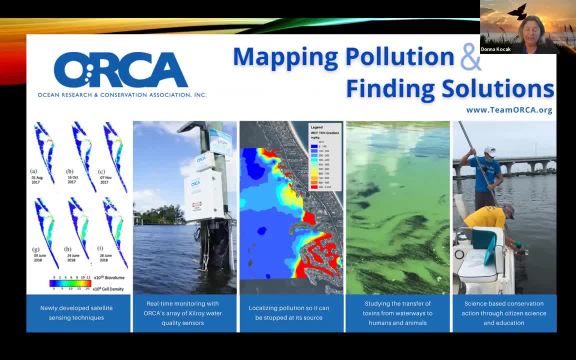 for Citizen Science in Vero Beach. They're expanding rapidly. They're training an army of citizen scientists how to identify problems and initiate solutions And over the last three years they have over 230 engaged participants and 480 recruited, But they've had over 3,500 students engaged. 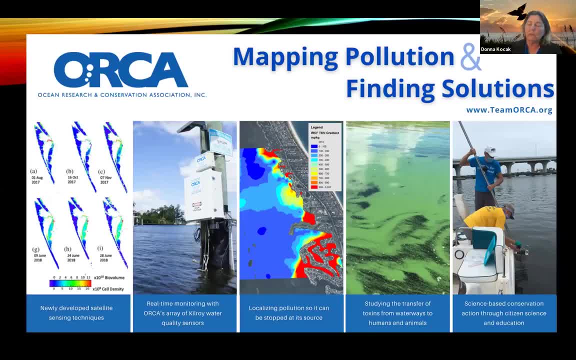 in data collection along the Indian River Lagoon. So this is one way. if you're interested in helping to clean up the Indian River Lagoon, this is one way all of us can get involved. Just stop at the ORCA's new Citizen Science Center in Vero. 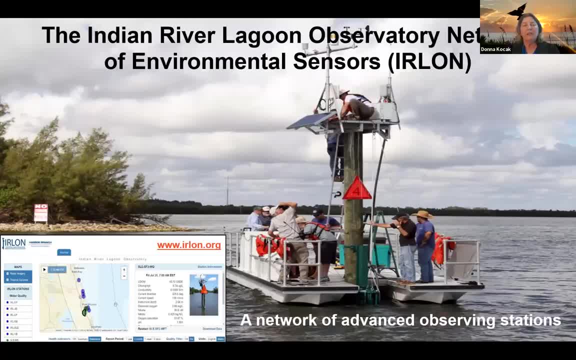 So another example which is right here, based out of Harbor Branch, is the IRLON Indian River Lagoon Observatory Network of Environmental Sensors. So this is a center headed up by Dennis Hanisak H-B-O-I-F-A-U, And it measures water quality. 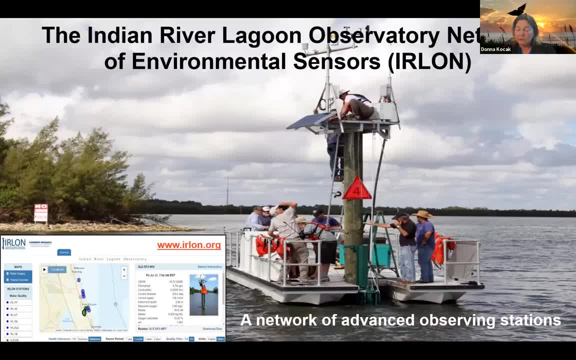 meteorological parameters, harmful algal blooms and coastal acidification. Those two last two are two things we're adding to the network, So data is streamed real time to wwwirlonorg And you'll see that the picture there going out. 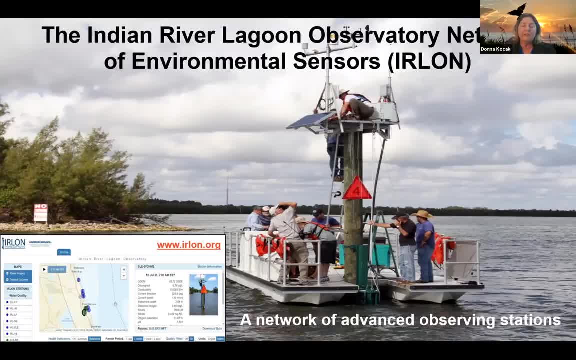 and maintaining one of the stations powered by a solar panel in the lagoon, Oh, by one of the islands. So all of these stations working together cooperatively and then adding, eventually adding other mobile platforms, is a nice way to monitor our lagoon and figure out. 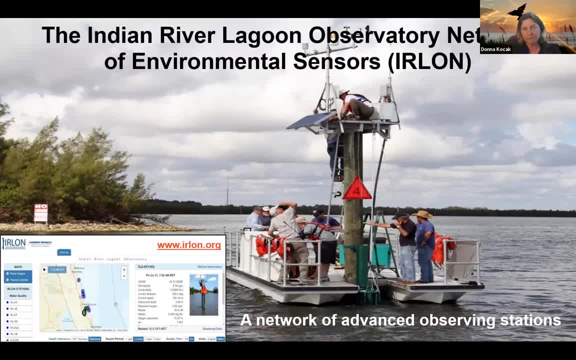 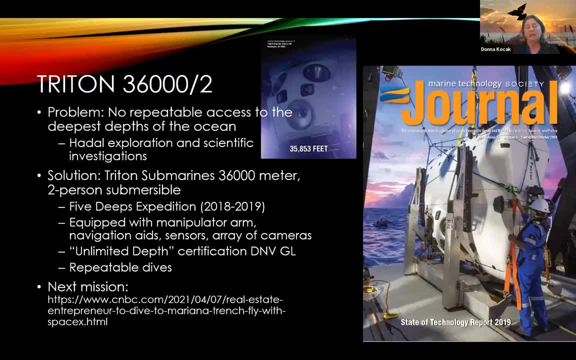 what's causing the pollution in the lagoon. So another local company I wanna mention is Triton submarines. Triton has recently developed a 36,000 depth submersible, two man submersible, And you'll see on the picture on the right is a submersible. 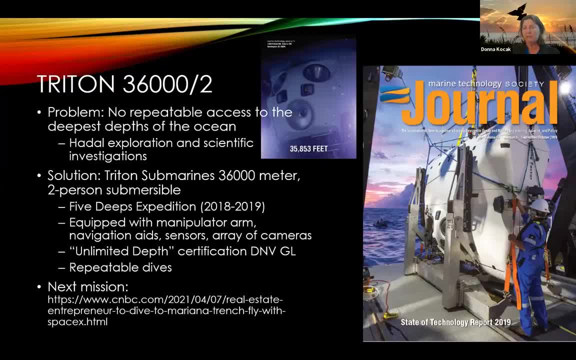 on a ship That was recently reported in the state of technology report 2019.. And then this: the deepest dive on that mission- it was the five deeps mission- was 35,853 feet. So the problem this is addressing is: there are no way. there's no way to repeatedly access the deepest depths of our ocean. There's a lot of exploration and scientific investigations that can be done in the hadal depths. Cameron went down most recently to the depths, but it was a one-time shot. This solution is Triton submarines submersible. 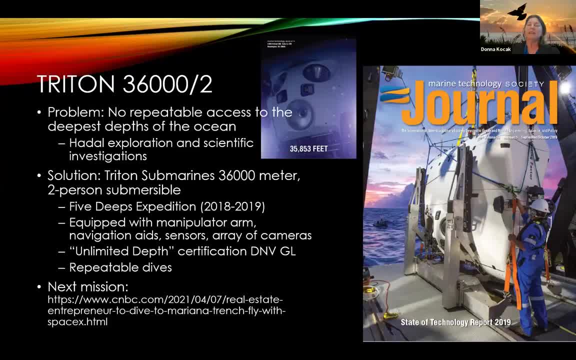 That was part of the five deeps expedition that I mentioned, but that can repeatedly go down to the depths, And they're actually doing that now. The five deeps covered the five deepest points of all five oceans, including the challenger deep, the Mariana Trench. 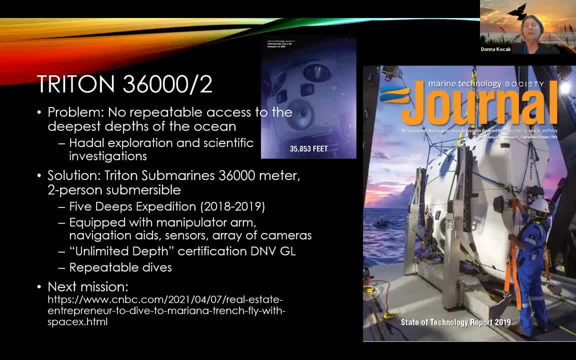 And that was the 35,853 feet. That was an 853 foot dive. They went on those dives between 2018 and 2019.. The sub was equipped with a manipulator arm, navigation aids, sensors and arrays of cameras. 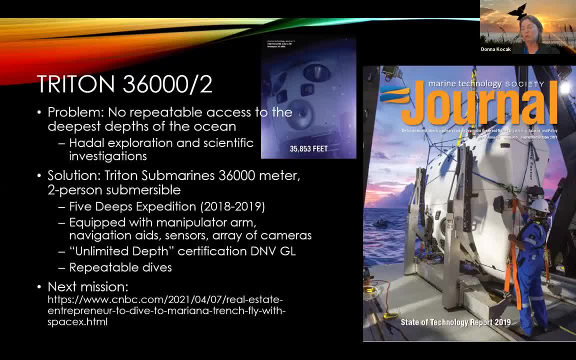 There were also landers that were dropped down there to transpond with each other and triangulate the precise position of the submersible at that depth. So they, the submersible, was giving an unlimited depth certification by the DNV GL, which means you know. 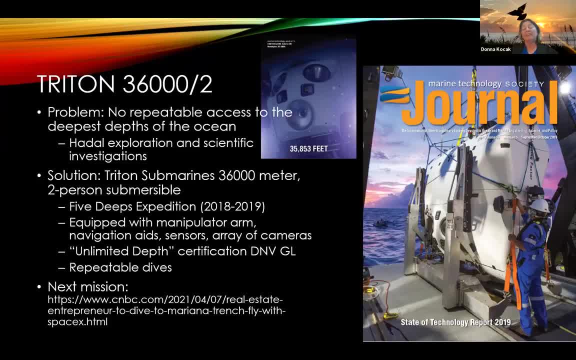 it's, it's. I don't know that there was another unlimited depth certification. I think it was the first of its kind, but it repeatedly dives down. So the next. I know Kathy Sullivan, an astronaut, has recently gone down in it. 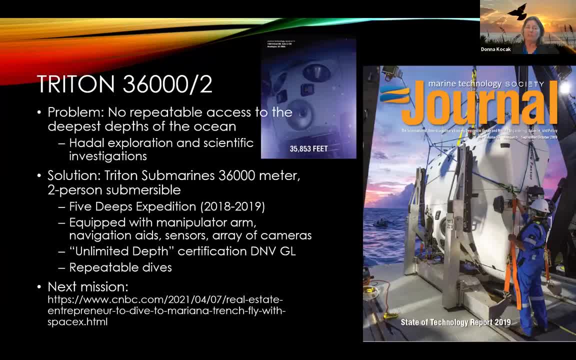 And there's been other other notable people. There's going to be the next mission coming up. There's a real estate entrepreneur who is actually going to fly on a SpaceX flight up to the space station And now he's going to be just before that going down. 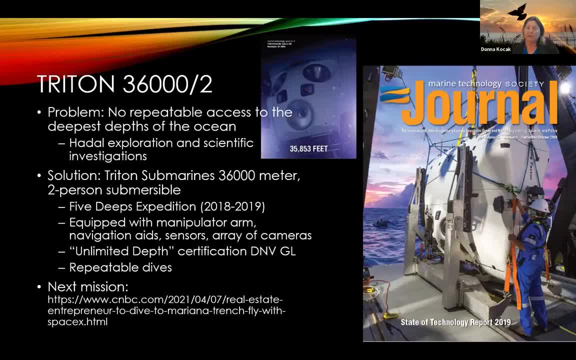 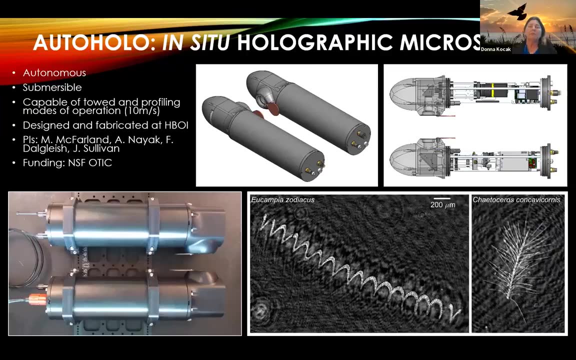 to one of the deepest dives in the ocean within a year of that space flight. So that's recently out on CNBC there. Another sensor that's local, from Harbor Branch, is the auto hollow, So it's an in-situ holographic microscope. This is capable of imaging larval. 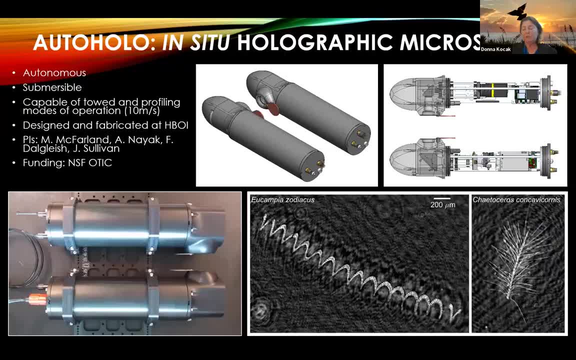 and invertebrates. It provides pretty accurate 3D information And the goal of the system is to actually be able to identify the organism real time using artificial intelligence algorithms, maybe neural networks, And this can be autonomous operation and it's also capable of being towed at pretty high speeds. 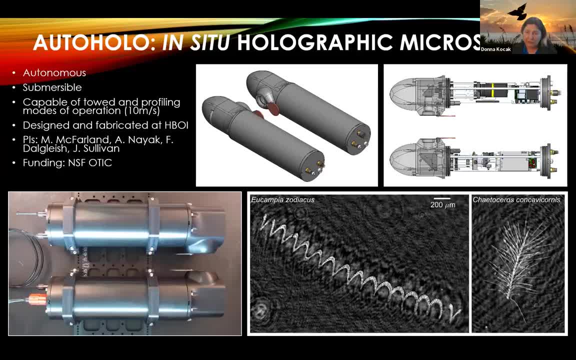 10 meters per second. the accuracy, the resolution and the is about two microns in size, so it can capture the tiniest of the critters. It's designed and fabricated by Harbor Branch and the PIs are Malcolm McFarland. 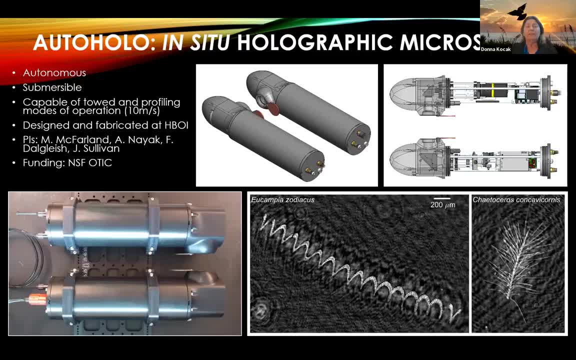 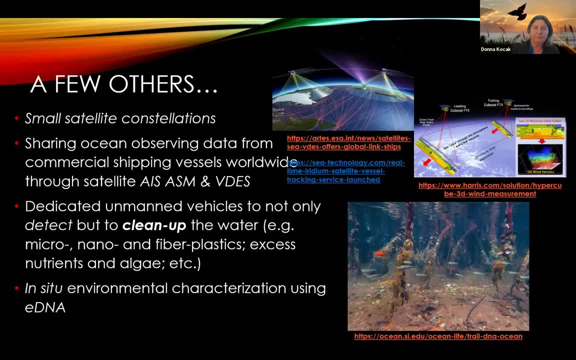 Eddie Nyack, Fraser Dalglish and Jim Sullivan, And this was funded by the National Science Foundation. So there's a few other that I'll just mention. I didn't put a lot of details here, but small satellite constellations. So currently we have a lot of large satellite constellations. 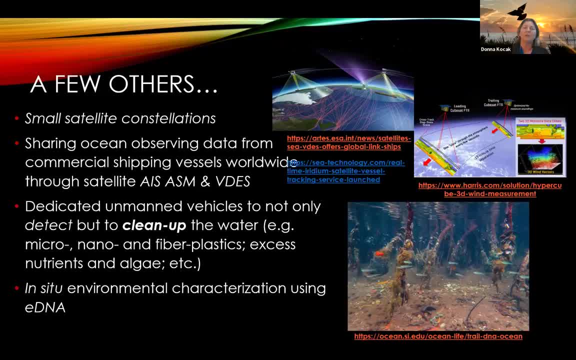 up there. but it's turning out that these small satellites can be launched much easier, they're more cost effective and they can actually perform missions in collaboration with each other. Put a little constellation up there and they can trail each other, and they hit points on the Earth faster together than one large. 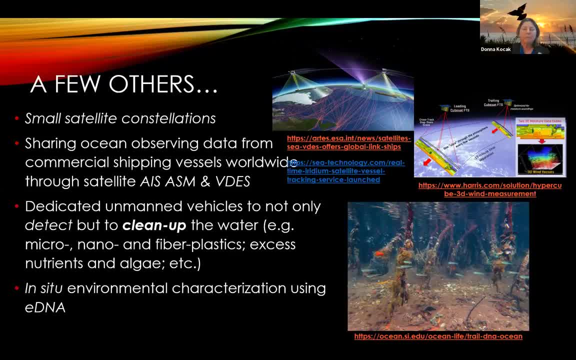 constellation. one large satellite would Sharing the ocean, observing data from commercial shipping vessels worldwide through the Satellite Automated Information System, the AIS system, where you can send data up. you can collect it from vessels of opportunity that are crossing the ocean every day. These could be freight ships or whatever. 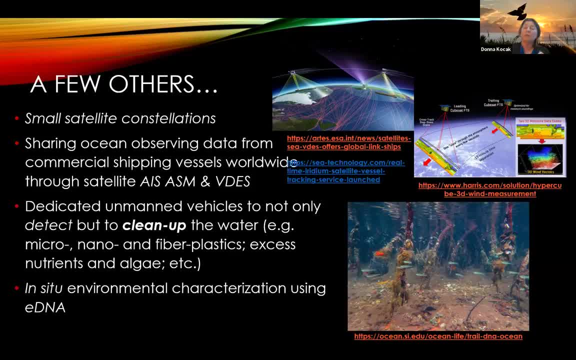 And they can have sensors on board that send this data up through the AIS, ASM and BDES messaging system. They get back real time. So that's one way of gathering data across the ocean, kind of comparable to the undersea cable method. The problem there is the calibration, You'd worry. 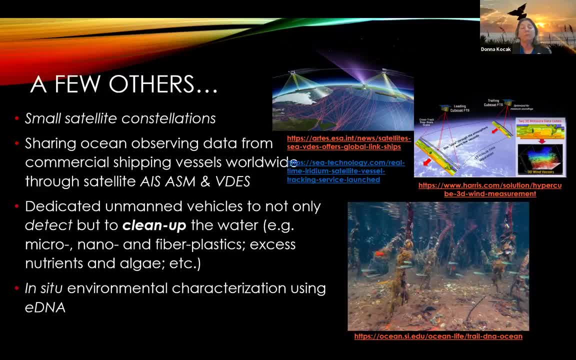 about: are the sensors calibrated? But that could be worked out. Another: in the future we're liable to see dedicated unmanned vehicles to not only detect but to clean up the water. So we talked about having a mobile detection network. Well, how about a cleanup network? 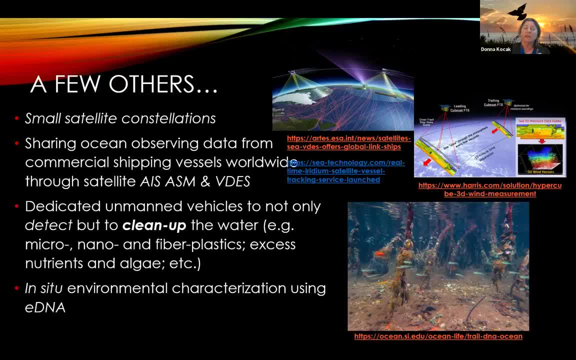 I know there's, I believe Harbor Branch and other universities are working on studying micro, nano and fiber plastics and how to remove them from the water, And there's also the problem with excess nutrients and algae. So you have, those are what's creating the ocean acidification. 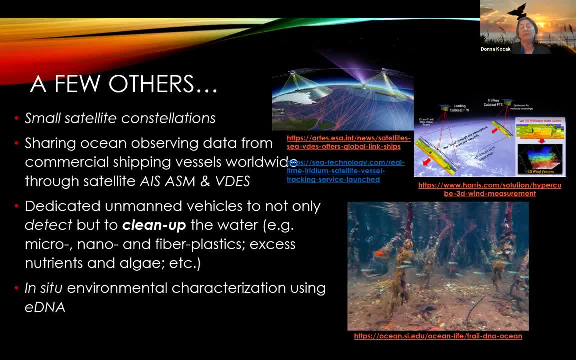 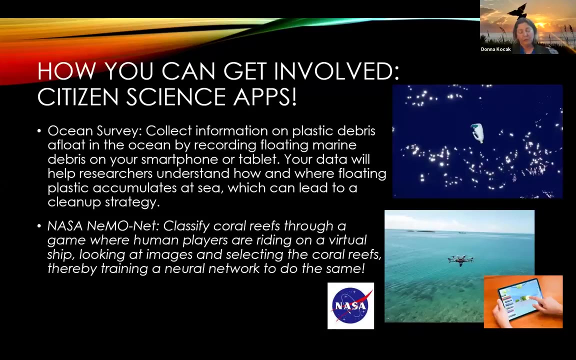 and the red tide, the harmful algal blooms, the bad algaes, And then the other thing, another technology that's up and coming is the in situ environmental characterization of eDNA, So the gathering the DNA from the environment. The last portion of the talk is going to be: how can, how can just everybody get involved, How? 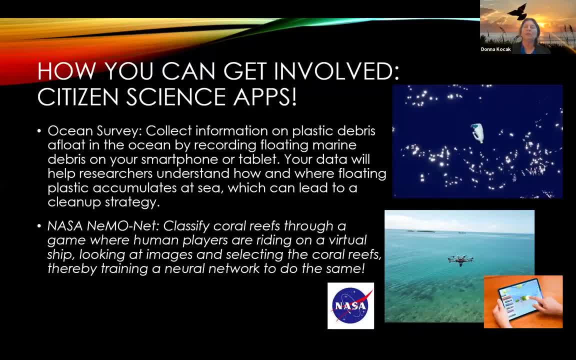 can you get involved, And the easiest way is through citizen science applications, And there's a lot of them out there. I researched this six years ago. there were a lot and just looked a whole bunch more up and there's even more now and some of the same ones are still there, so they're really easy to use. you can load the app. 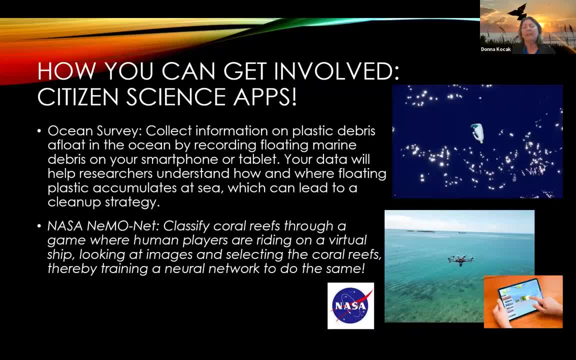 on your phone. one of them is ocean survey. so if you're out in the ocean or out on the river or any kind of waterway at lake and you see plastic debris floating around, you can take a picture of that. then your gps time stamp and time stamp will document the location and time of the 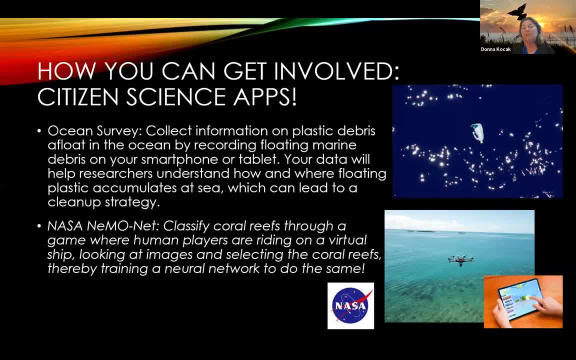 of the event and send it in, and this is going to help the researchers understand how and where floating plastic accumulates at sea, which can lead to cleanup strategies for our rivers and oceans and waterways. there's a debris tracker is another one that's around. it does the same thing, and 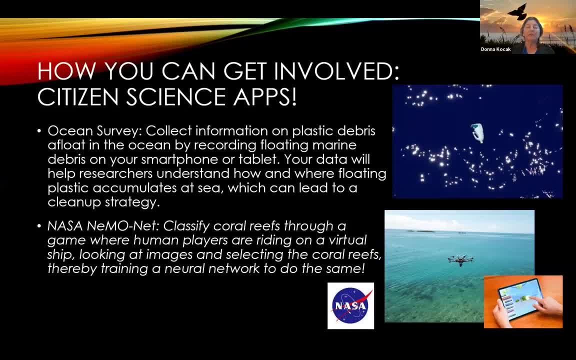 there's also one specifically that's designed for rivers- river trackers. another one by nasa- and i was surprised to see this- is a nemo net. so this is a really, really slick concept. it classifies coral reefs through a game. so the human is a player in the game and you're. 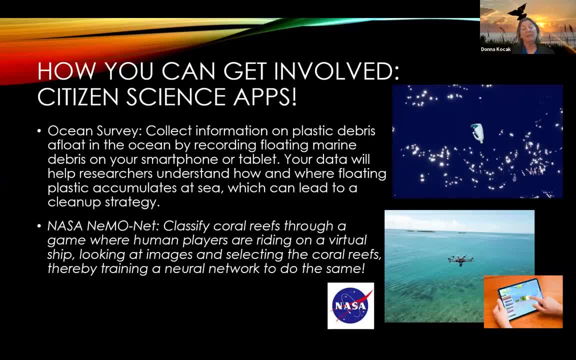 riding on a virtual ship and you're looking at the images that's being collected underwater underneath the ship and from that you're simply selecting where the coral reef is in the picture, sort of sort of like when you have to identify the signs in the picture to get it in. 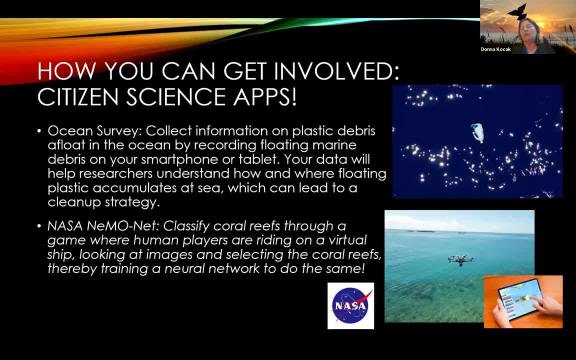 but what it's doing is it's learning. uh, there's a neural network learning how to identify the coral reef from your decisions, so you're actually providing information. neural networks have a hard time identifying the data on their own, but given the way you approach solving it, they can learn a. 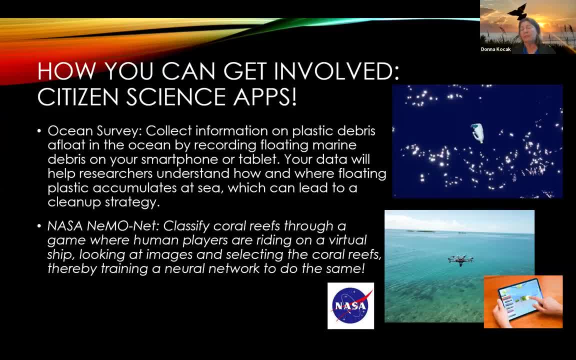 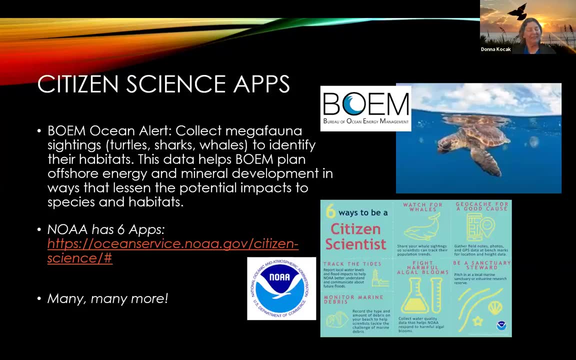 lot from humans. so a lot of the data is collected very cheaply through drones in shallow water and then you just run that and have volunteers solve the problem. the problem for you train the networks. so some more citizen science apps. there's another um, boehm. boehm is the um. 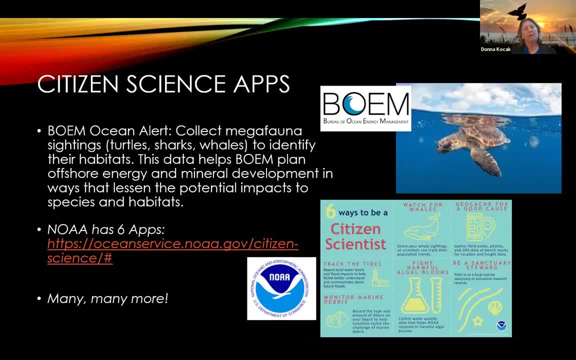 gosh bureau of ocean energy management and they have one called ocean alert. so a big problem in the oceans, whenever you're doing any kind of oil and gas deployments or servicing, is looking for marine mammals that you can only ply or like your ownelled on the surface or under the water. 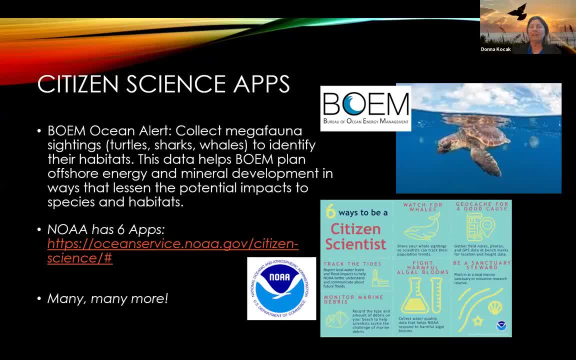 um, so you want to try not to interfere with them. so they have a an app called ocean alert. it collects the megafauna sightings, such as you know, turtles, whales and sharks, that you report, and it'll identify their habitats where they're found. so this data helps them plan offshore energy and mineral development in ways that lessen the. 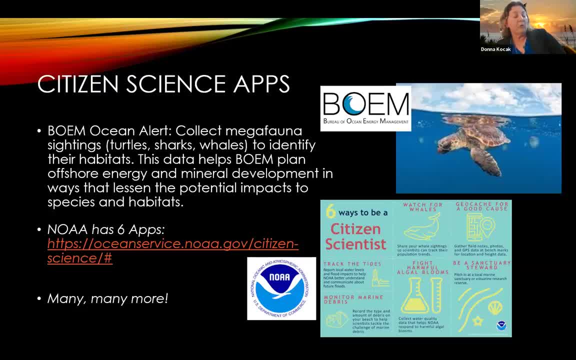 political or the potential impact to species and habitats. so by collecting thoseägbs and networking materials, collecting this data, they can figure out where the whales are. They can also do it on a timescale over long periods of time. And another- I'll call six apps- is NOAA. They have a bunch of them listed here. 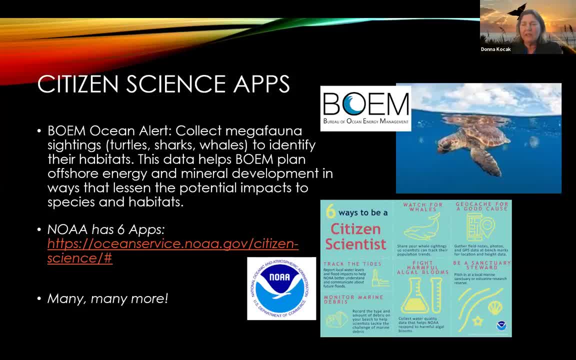 There's track the tides, monitor marine debris, watch for whales, geocaching, fight home for algal blooms and be a good steward of the ocean, So they have many apps there that would be interesting. There's many other ideas that are out there on your phone, So it's a nice way to contribute. 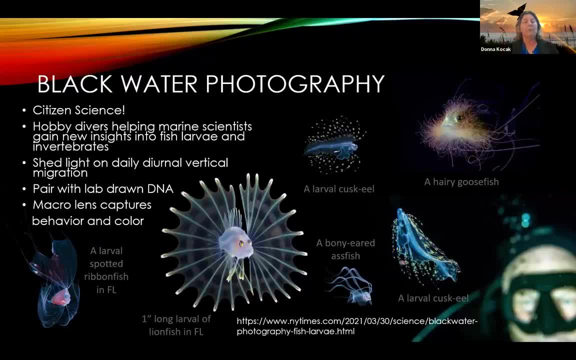 Finally, I'm going to summarize with my favorite method here. Makes me want to go get a nice macro lens for my camera. This is called blackwater photography, And Dr Frank, who used to be at Harbor Branch, pointed this out to me. 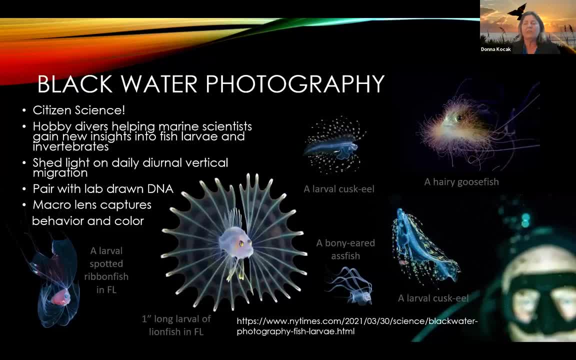 It was in a recent article, March 30th, in the New York Times, And it's about photographing larvae and invertebrates. It's similar to the hologram camera, but not because you're not getting any 3D data or anything. 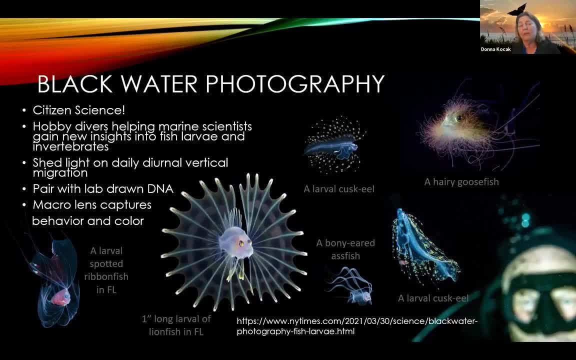 This is just looking at the larvae with a regular camera with a macro lens, But you're able to capture the color and behavior and location of these invertebrates and larvae. So hobby divers are helping marine scientists gain new insights into the ocean And I think that's really important. 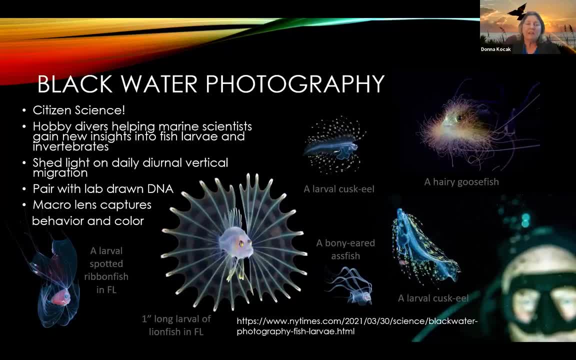 Thank you. Thank you, Lovell, And I just want to take a quick break, which is a great way for us to go with this last recorded session on archaeology. So I think there's a lot of information there. We're going through a lot of technical stuff, but I just want to make sure that we're getting as much data as we can, as we can. 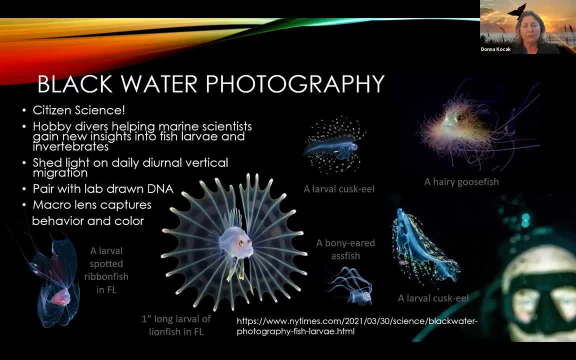 And I do want to pull up some photos of the work that was done with the NASA, Un破, taker and some other studies that we're doing with Attica in the Arctic. that, I think, was The person who started this. was from Hawaii And he just went out diving every night, started to take these pictures, beautiful pictures. 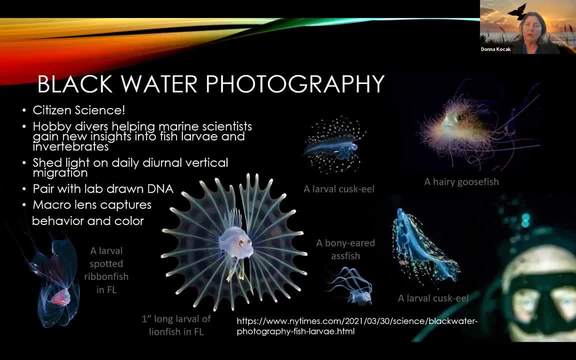 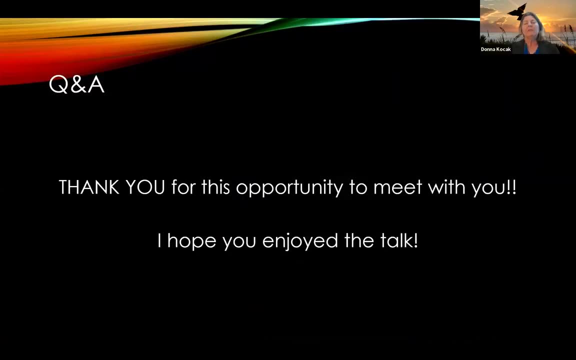 So what they can do to the researchers: compare that with lab drawn DNA so they have a nice identification: the color and the size and the or the color and the shape that goes with the DNA. So I know I'm just a tad early about what I thought it was going to be. 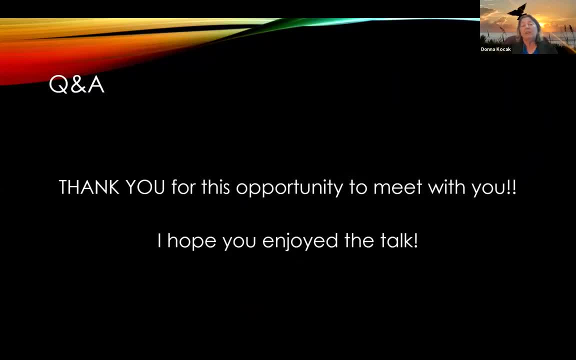 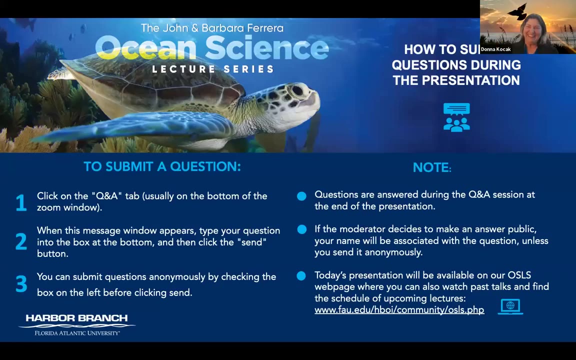 But I do thank you for this opportunity to meet with you and tell you about the decade and how all these technologies might help achieve the goals of the decade, and I hope you enjoyed this talk. Thank you, Donna. if you hear everybody clap, as you hear me clap maybe, Yeah, it's strange, virtually, I'll admit. Yeah, it's totally different experience. 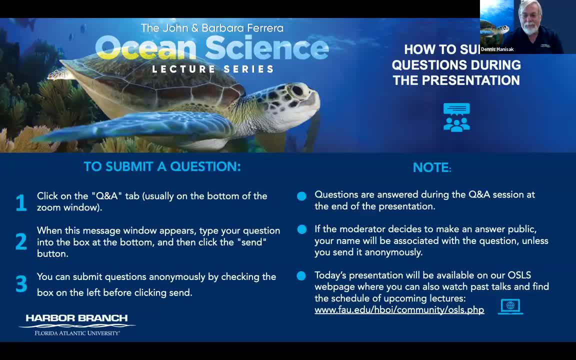 But I would think you know somebody so into technology would Would be okay with that So the audience knows. I think if you've done this before, Please type your answers- are sorry, your questions- into the q amp a box And I will moderate that and throw some questions to Donna. 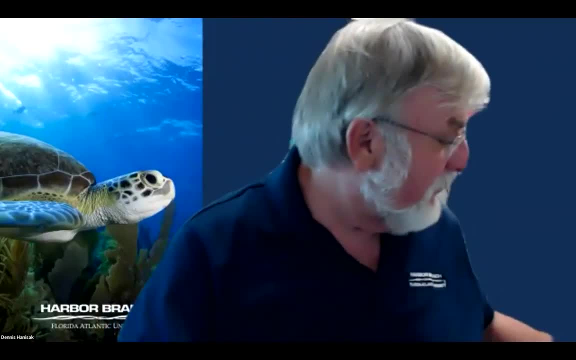 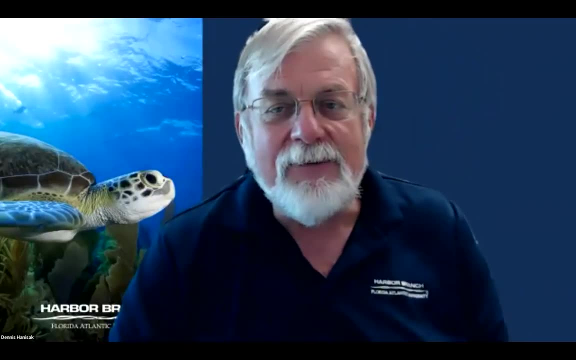 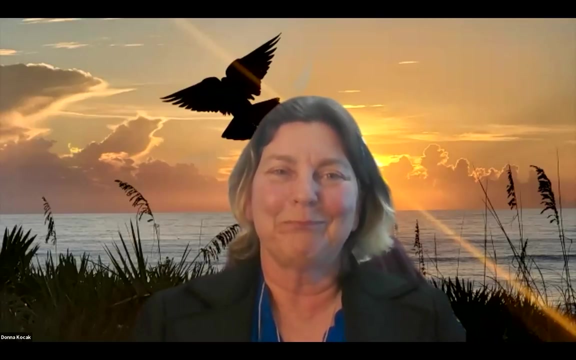 And while things are waiting for some things to come in, Yeah, Donna is some really interesting thoughts about future use of technology. So one of them: Yeah, Clean meat technology. Yes, So obviously you thought a lot about these things in the future. 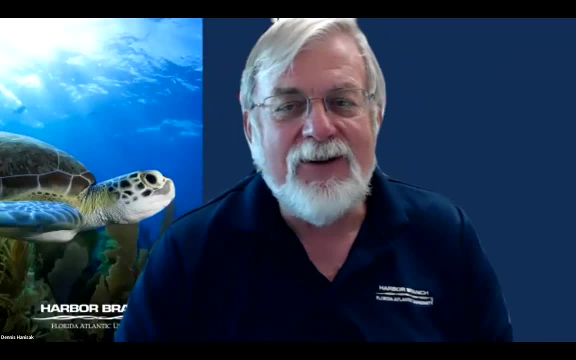 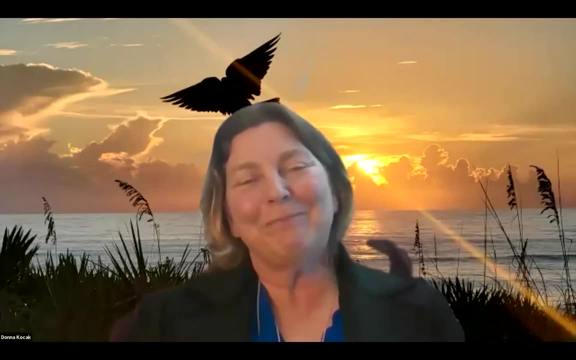 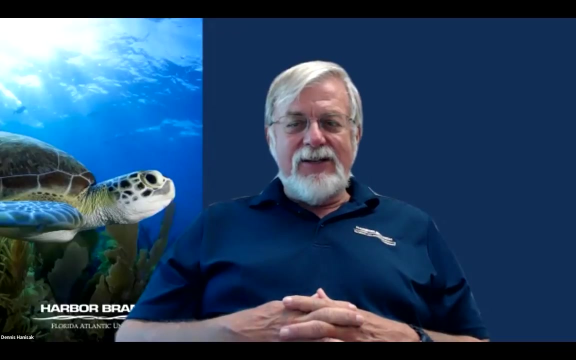 And you know you did wonder how long it would take for people to adapt to the idea that meat could be grown- really grown- in a dish. Yeah, You pointed out some of the advantages to that in terms of not having some of the contaminants and things that people worry about. 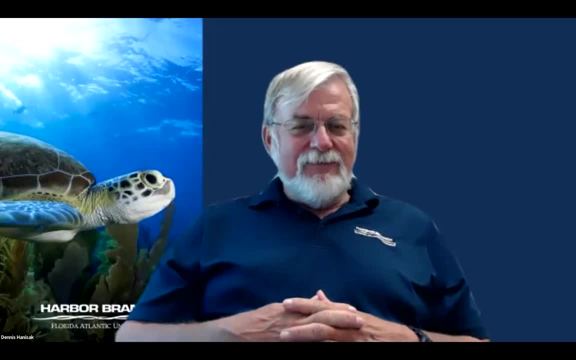 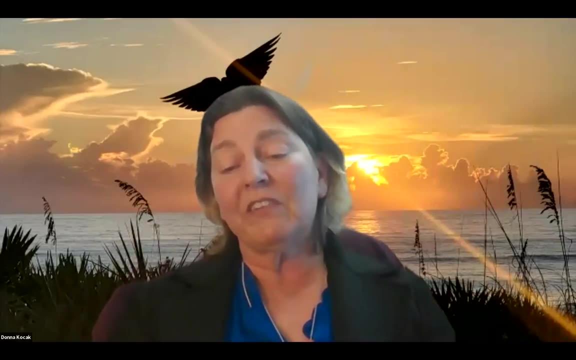 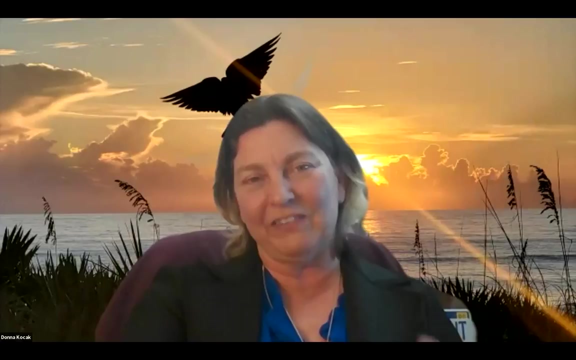 How far in the future are we talking? Not far So 2017. was that the finless fish? that was the first one. The problem is, some of these things cost, you know, thousand, hundred, thousands of dollars, or $10,000 for a piece right now, but that's because it's so new. 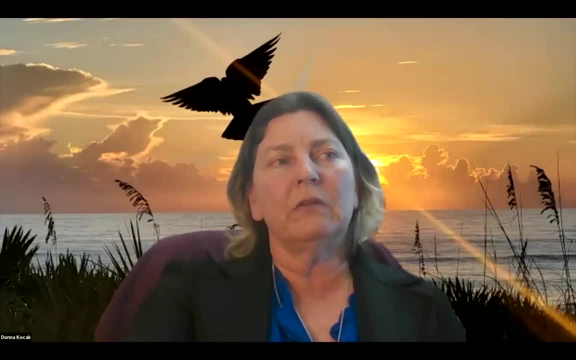 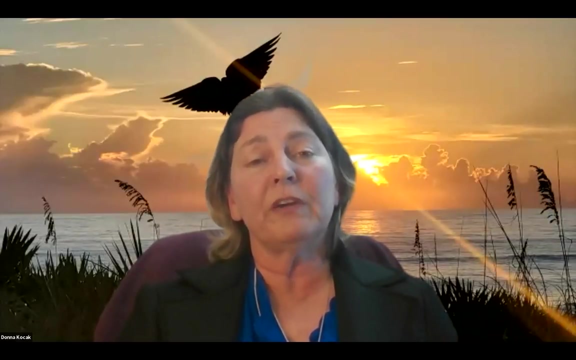 I know, you know, White Castle started out that way with or beyond beef, with its plant based hamburger, you know. but now they're doing it with it. you know this clean technology, This clean technology with meat and fish. So there's a. you know we're not talking very far. 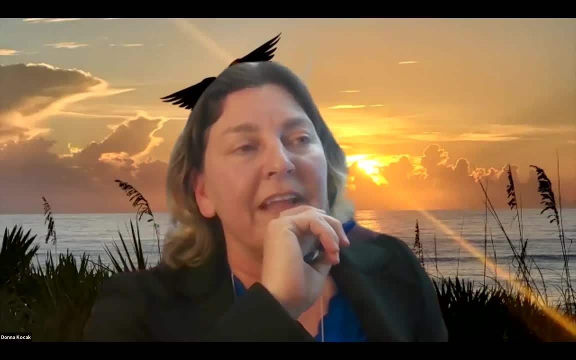 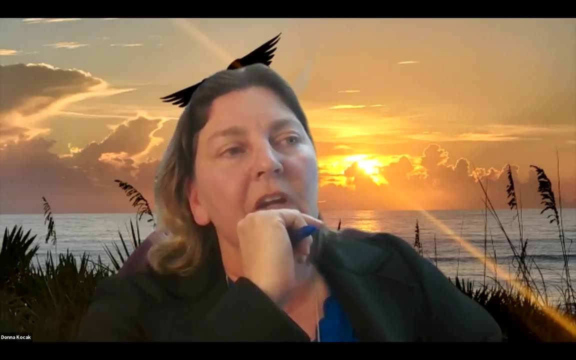 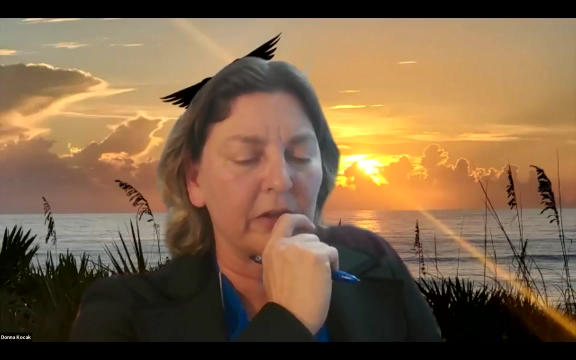 Actually, while the beyond beef- it's interesting, I just look them up and their plant based. so they actually just got into a whole bunch of new grocery stores across the country This year and they started out. Gosh, when was the IP? it was a while ago, but it but, it's, it's in, it's in the near future. 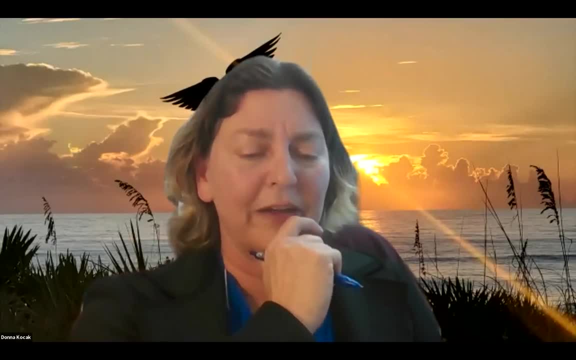 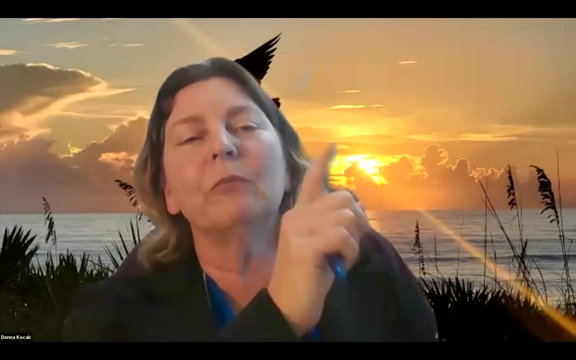 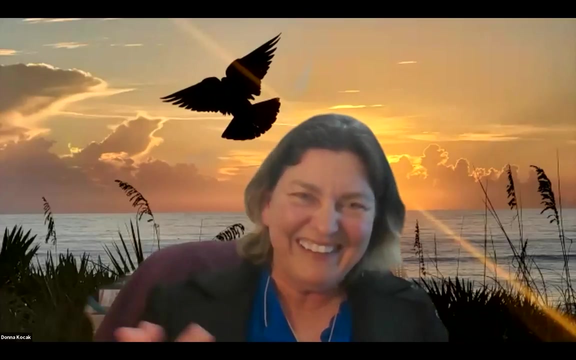 I have to have that looked up here. It's somewhere I see. I see another questions come in, but let me ask a couple more. give people time to type something. Well, what's interesting to what I like to say about that me? when I first heard about it they said somebody said 3d printed fish sushi. You know, I guess, what they do. they harvest that cell, they grow that cell, but they need to grow it on some sort of lattice because you need to grow the shape, So they can 3d print some sort of. I don't actually know how it's done. that's how I envision it. 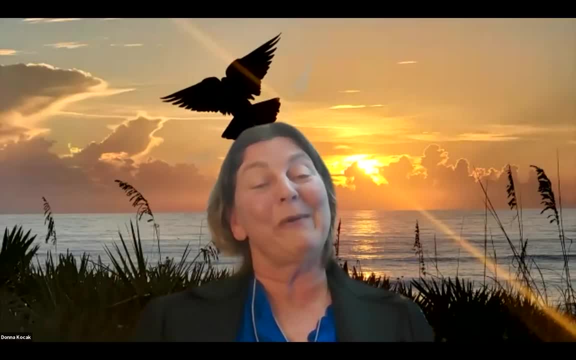 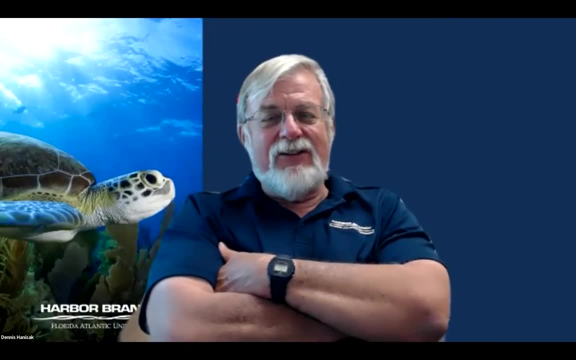 But whether it's really accurate, Yeah, I don't know, But you know that structure that we go on, So it's pretty interesting. Well, it's kind of funny. you bring up 3d printing, because that's another technology that I think initially we thought was kind of a curiosity, but it's not. 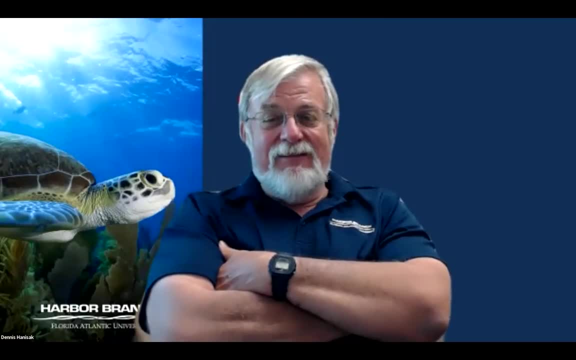 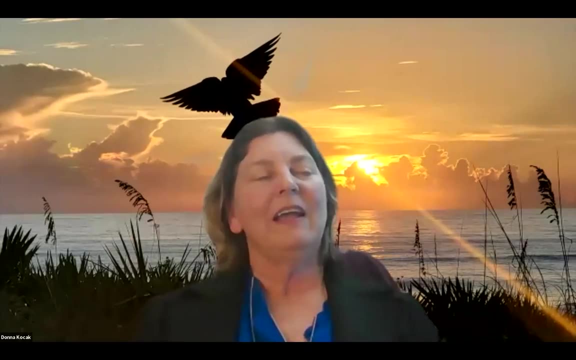 Yeah, I mean it's used in all kinds of applications now. Yeah, And it can be done anywhere, can be done in somebody's garage or living room for them. It's actually saving the, the Navy, a lot of money. they're putting them on ships now. 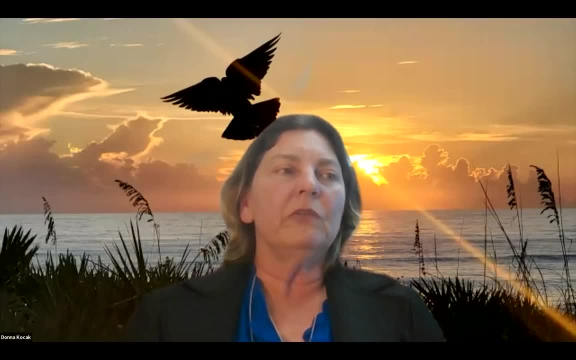 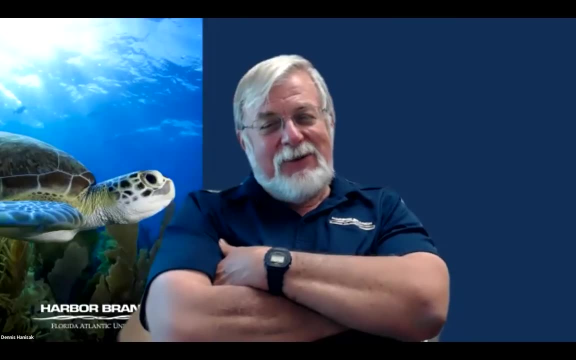 So if you don't have a spare part on a ship and you need it, You're out at sea- you print it. So even if it's a temporary face, Well, we sure could use that in the old days of when we had ships, huh. 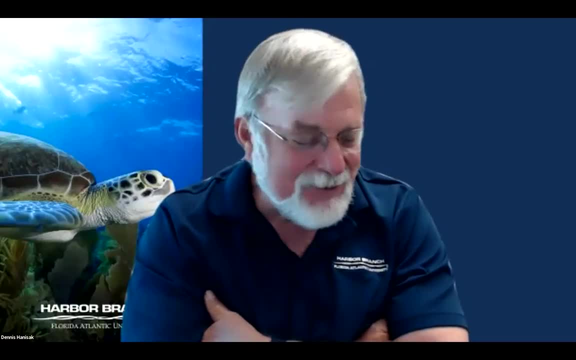 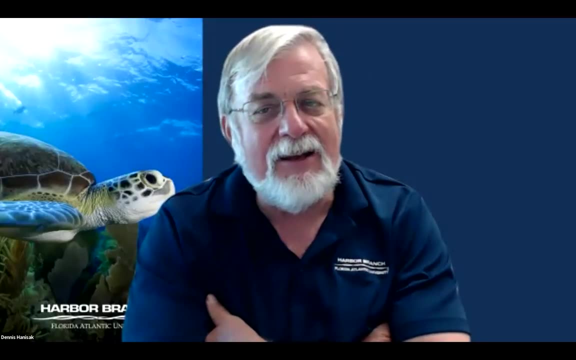 I always have to go important wait for it to get shipped from England. Yep, That's true story. So another one was: you know, these marine vehicle highways, that kind of thing idea too. so one thing I wondered about that: A lot of that, I guess, would be probably eventually be an international waters. 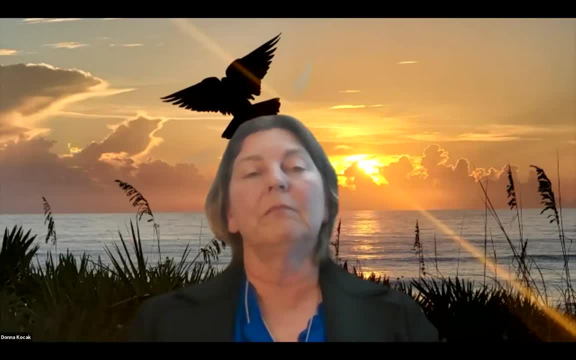 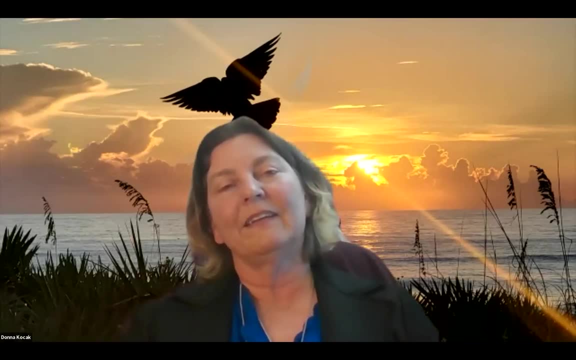 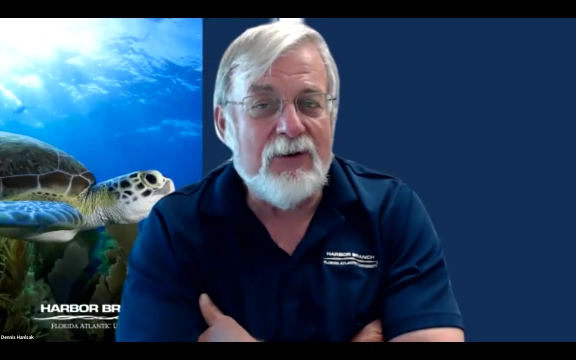 Great, Would you think? Yeah, So so is there going to be, as part of this UN decade, is that part of trying to get countries to kind of work together and deal with that, because you know it's so hard to agree to do things that you know our international waters or or or or. 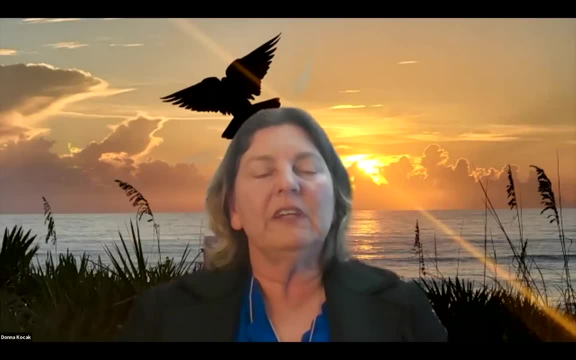 certain other parts of the world that are shared Absolutely. That is one of the biggest goals that they're striving for: to get members from every nation. So you know we're just succeeding quite well and getting getting people and then helping out the third world under underdeveloped countries with some of this. 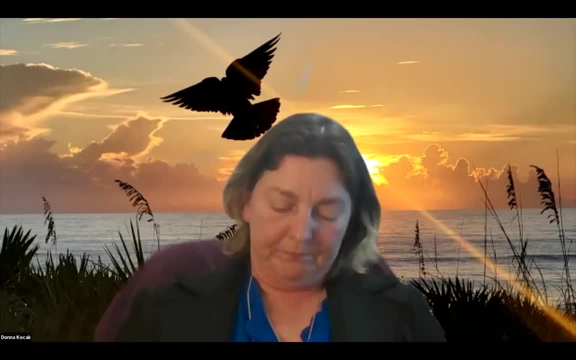 So collaboration is a big part of it. Going across These is always hard. there's always, you know, you have floating booze, the Argo boobies- floating between countries and around the world gathering data, and those were questionable for a while to you know. could they be floating and gathering data? 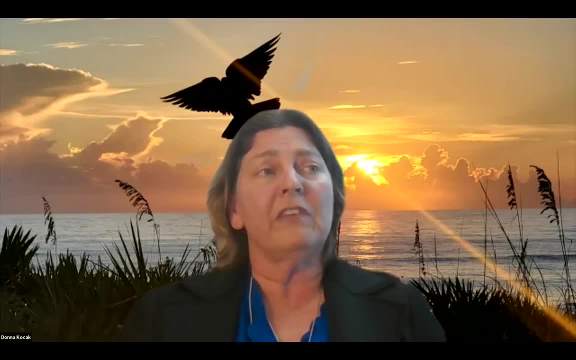 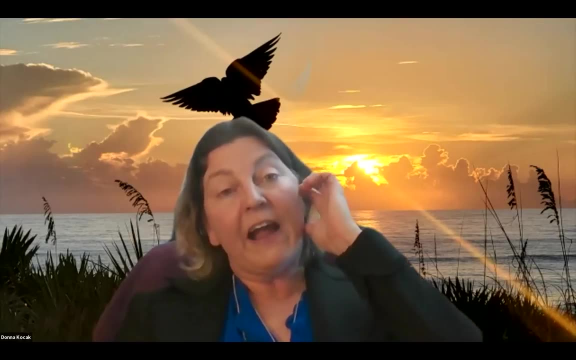 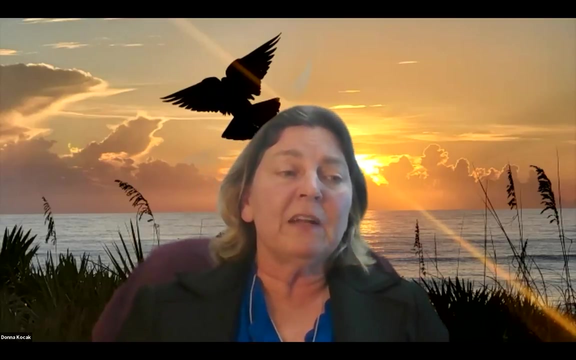 So it's similar. there will be similar issues and, And they'll have to be, policies about that. But that's another area to you know, with the, with the printed, with the cellular agriculture, Right, you have countries who really survived by fishing. But if you think about it, if the modern culture or, you know, forefront countries would go to that agriculture. 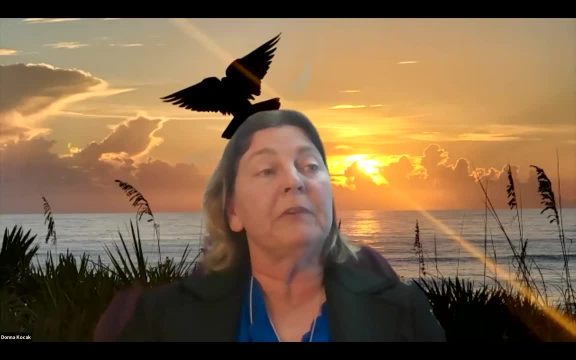 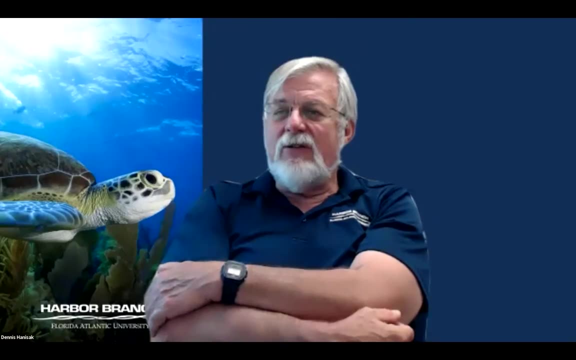 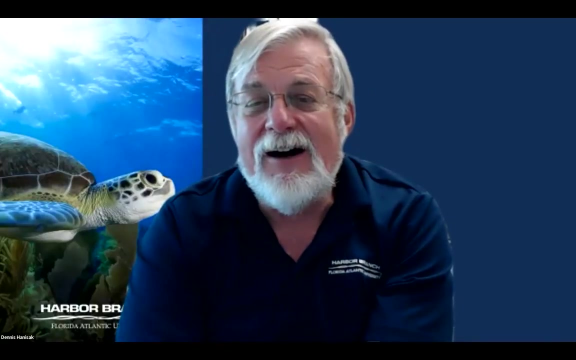 You could still have some people fish, you wouldn't have the overfishing population and you give things a chance to come back and survive. So you could do that, So you could gradually wean off of that. Okay, so one of the questions we got in is from is from Reg Jones, and Reg is one of our readers. that's always good to see you in person or virtually. 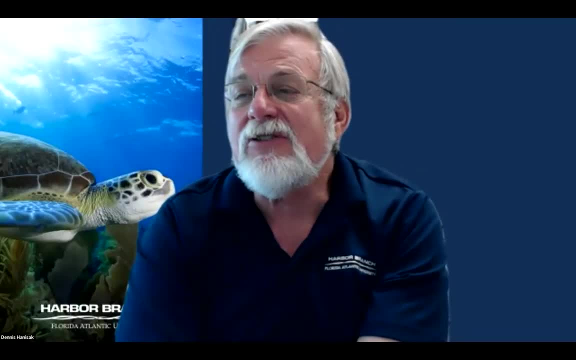 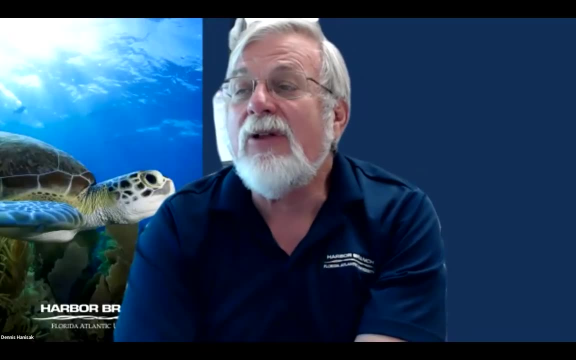 And I hope you're doing well, Reg- and your question or comment. I think it's a comment that evokes a question, so get your thought on it. You talk about locating plastic collection spots in the ocean So the cleanup efforts can take place. 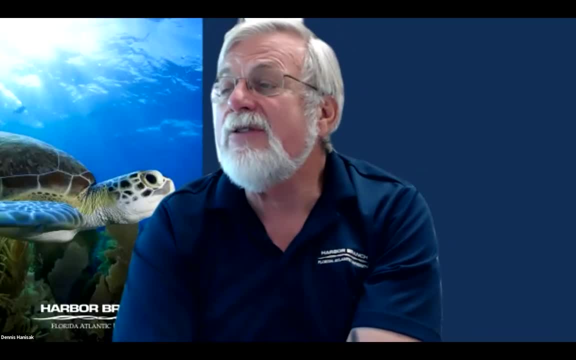 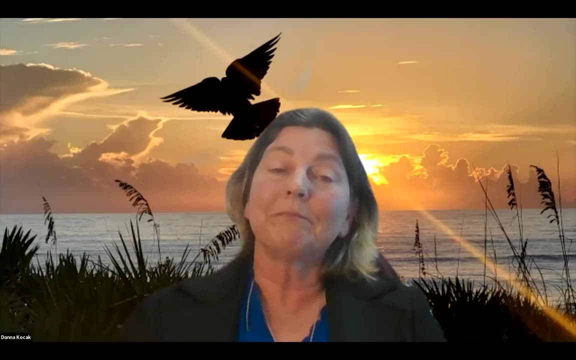 So his point is this is the problem is is more one of production rather than if cleanup. if we do not stop production right and overuse of plastic in the world, we will never catch up in a cleanup process, and of course, that said for a lot of other pollutants. 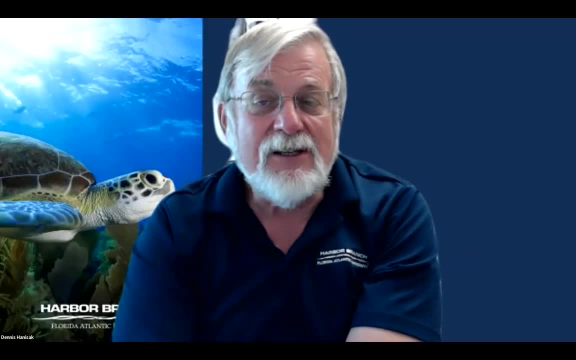 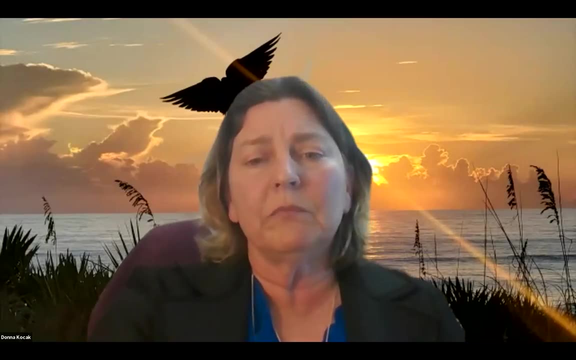 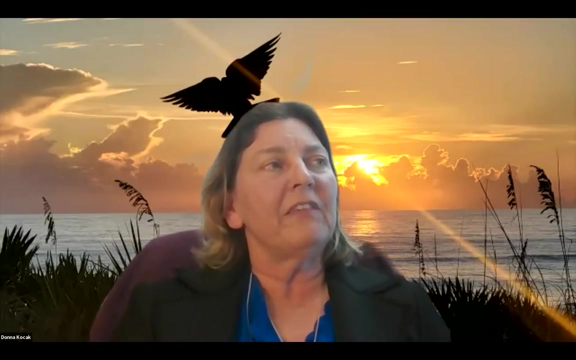 like nutrient pollution is better to catch it at the source. But anyway, do you have any thoughts? to Reg, Yeah, absolutely, Absolutely, And I think. I think that my video cut out. Oh no, there we are. I think, as we learn more about the potential plastic effects on us, you know, I think we're it's really going to seriously make us stop using plastic. I've got friends who won't use it. you know, get the, get the glass bottles. 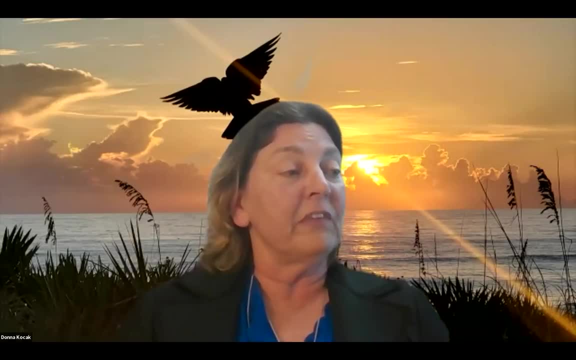 recycle the water from the glass. just let's just stop it. it's going to take, you know, packaging now the packaging of commercial microwave dishes and things like that is really got to stop. But but you know, you see the trend, they're going to. 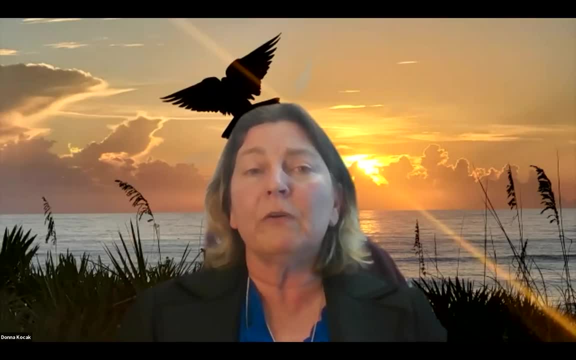 Some of the places are going to paper straws now. you know, some of the Starbucks or some of those other restaurants are doing paper straws for recycling. so you know, I think it's just going to take a mindset to do it. But absolutely, you know, maybe, maybe, once we stop them, maybe we can catch up. 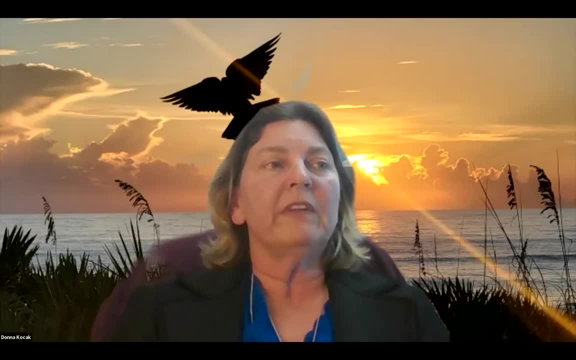 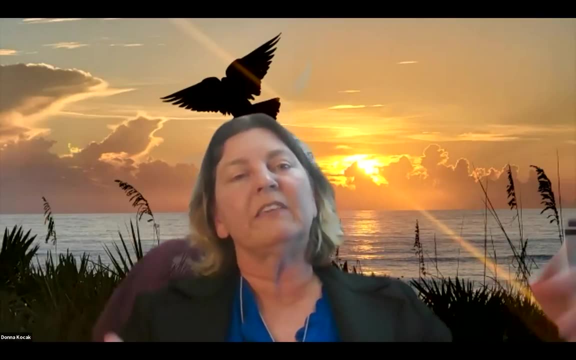 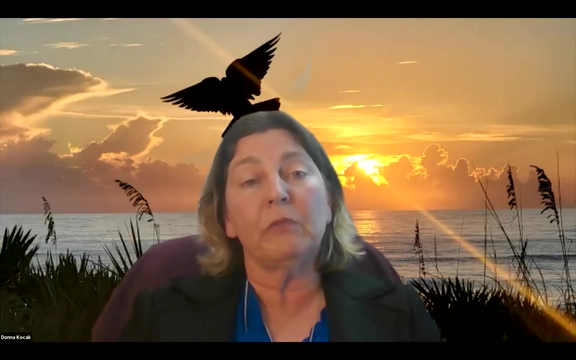 And I think, having a bunch of autonomous vehicles running around, whether it's it's air drones or whether it's underwater vehicles or surface vehicles, you know they have that big giant to from Hawaii that they try to get out there to collect that pollution. So you know we're going to try and you know, have these things unmanned doing all that, you know, as long as they don't interfere with the animals. 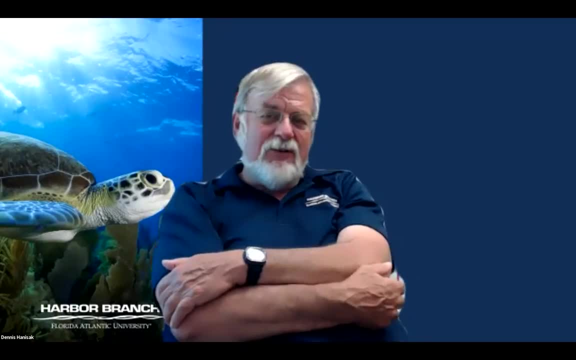 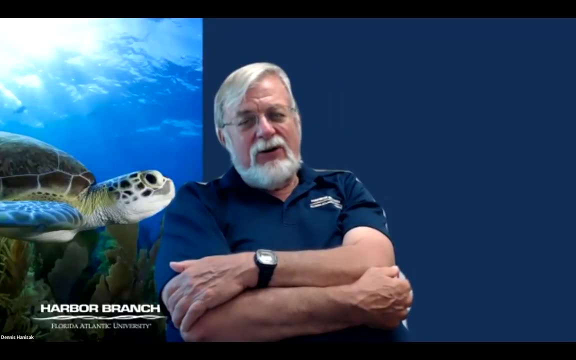 See. So you think that's something you and would would want to get out again. I mean, the question is that a lot of that you know, when big garbage patch, For example, they're in international waters And yeah, you know. so I mean the question in the end is gonna be who pays for it? right? so I don't think it'll be. your in your in your work, do you get into that kind of question? you get into 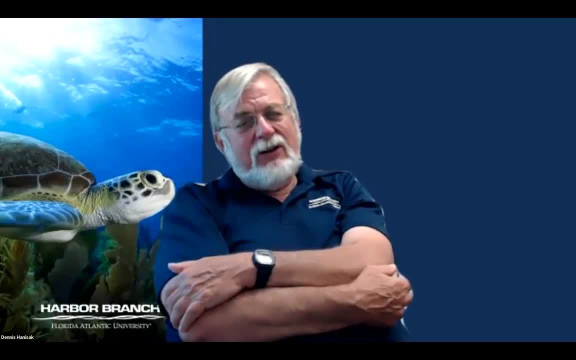 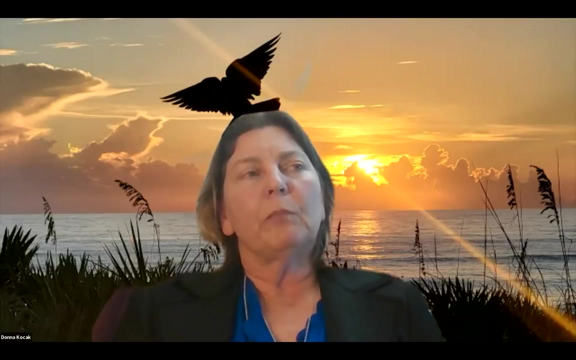 Yeah, you know, when you work on this UN task force that you're on and other things that you do, It's just evolving, So they're going to have questions. There will be some money for programs but there probably won't be a lot to support all new technology development That'll. 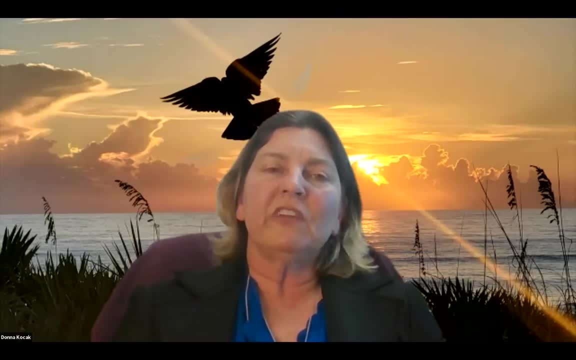 probably come out of another bucket. I think they're going to start with trying to educate people and looking at collecting data for policymaking. You know, mapping the oceans is a big Seabed 23 is a big goal, So that's definitely there is money for that. 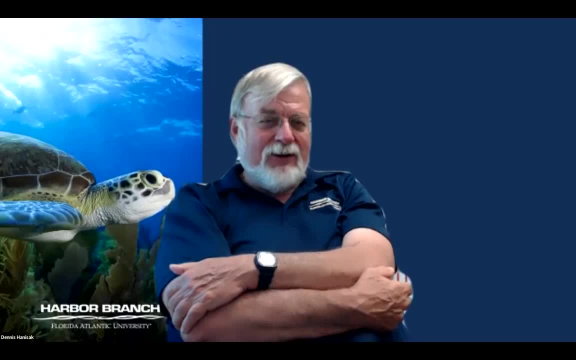 So you say it'll come out of another bucket. That'd be like a metal bucket, not a plastic bucket, right? I hope so. A piggy bank, Yeah. So hey, I got another one for you, So I was really. 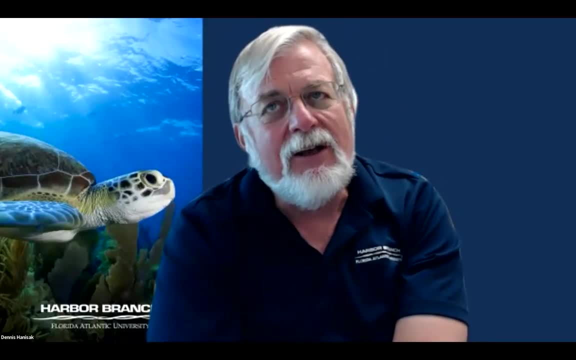 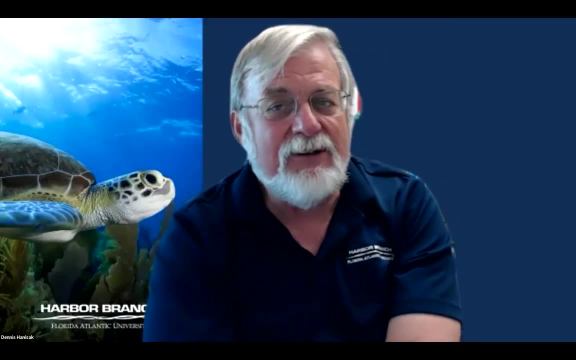 glad that you talked about Triton And you know there was a lot of people that used to work here in our submersibles that worked there And you know it's nice that you know Triton is right here in our local community and they have done incredible things. 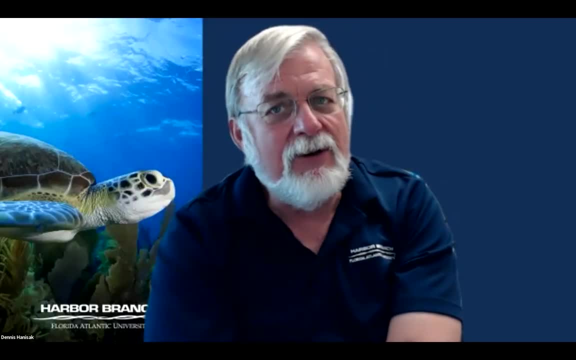 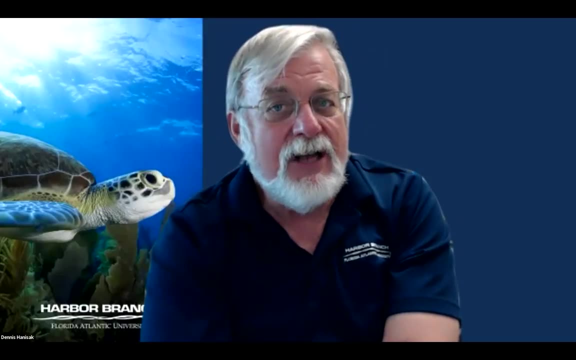 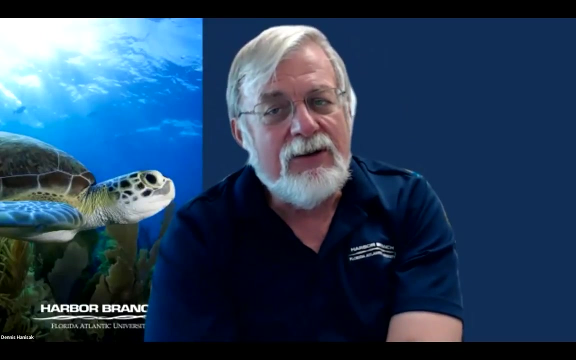 You know. so much of what you talked about, though, was: was, you know, not not with human humans actually going underwater, And, of course, a great part of our legacy here at Harbor Branch was the human occupied submersibles. Now we don't do that anymore. You know, we stopped in 2010.. And 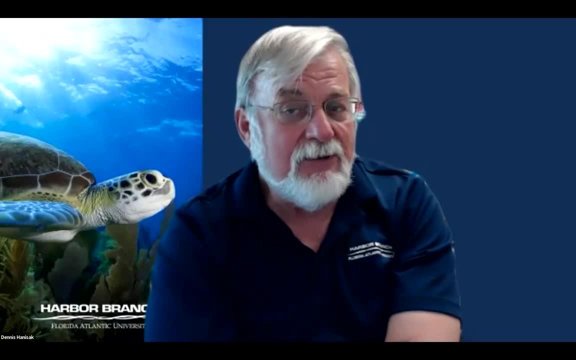 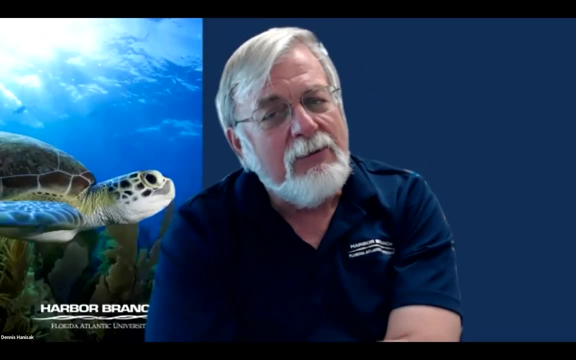 one of the reasons was things were changing and the economics didn't work out for that. Do you, do you ever See that much need? I mean, the Triton one is kind of one of you know pretty pretty I mean. 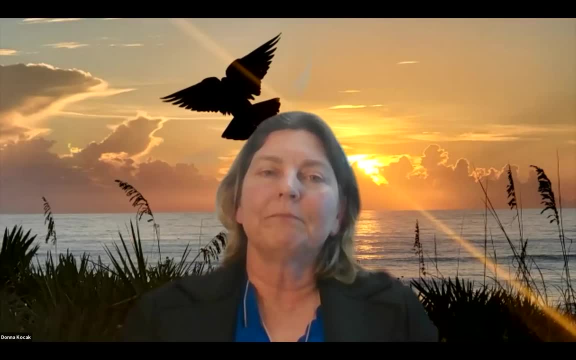 it's kind of what they're doing. It's kind of a niche thing right now, Yeah, But do you do? you see? I mean, at some point is there any need for us to think more about we being, you know, the? 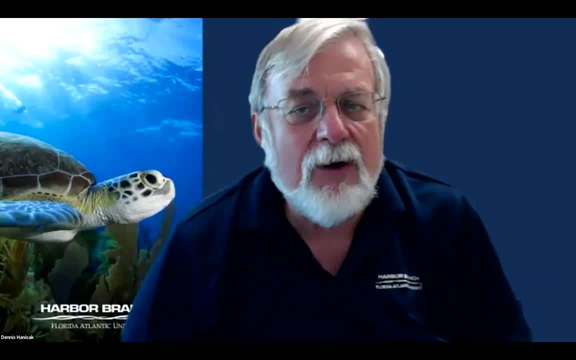 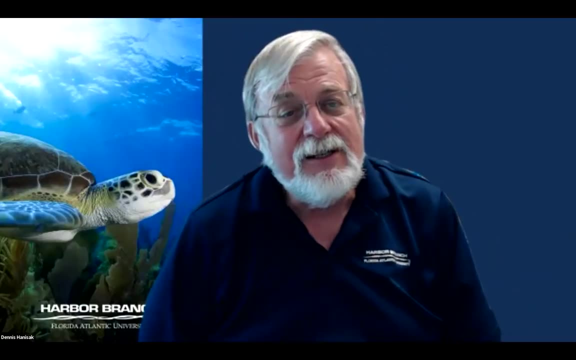 whole, the whole, not just Harbor, not Harbor Branch, but you know the broader we. is there a reason to think that there's a place for humans to do this? I mean, it's a whole different experience. Yeah, it is a niche to do that. It's a niche. 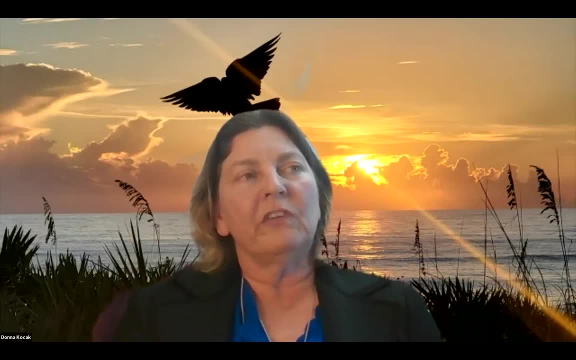 But I think you know right now what Patrick's doing. it's more becoming a- I don't want to say entertainment, but you know- kind of like a tourism kind of niche now. However, yes, I think there is a niche, a need, And actually if you think of the DOD world, that goes down a lot deeper. 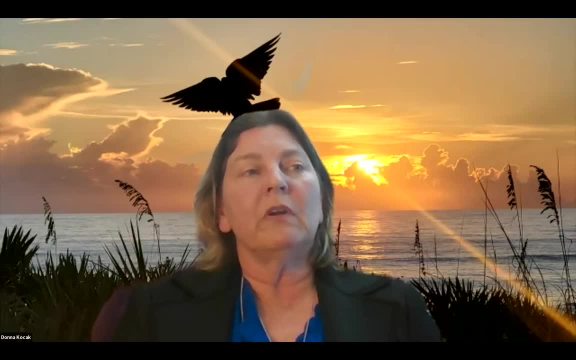 than any other man, things that go down, you know. so there, as in the DOD world, things are going deeper. So, as you know, I think, I think you know we'll go down and see things. But even science, 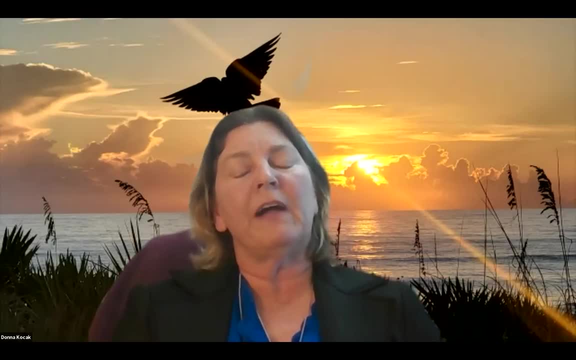 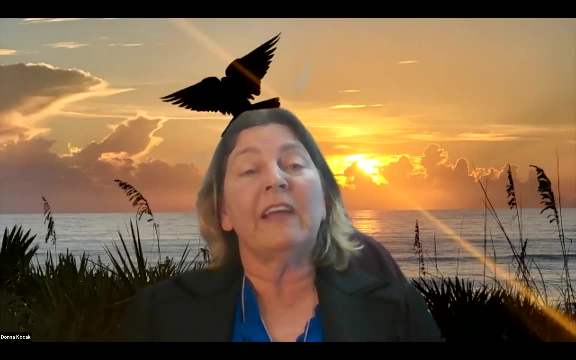 I think it's important to get down there. What one, a couple of things Patrick found, sadly. they found a plastic- it was either a bottle or a can- down there near the Mariana Trench, you know, sadly bad. And there was also a small, you know, cable, fiber cable down there. I mean it's you. 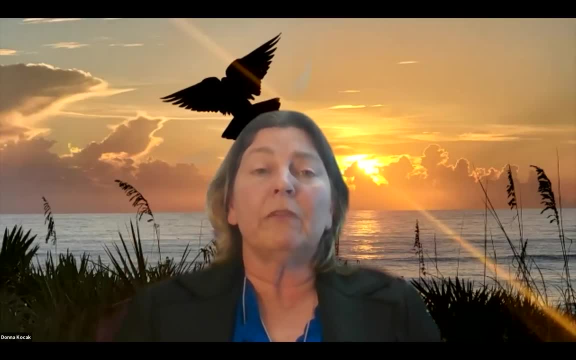 see all sorts of things down there that it's sad that they make it that far down. It's pretty true Any place we've done any recent ROV work or when we used to do submersible work. I mean it was. 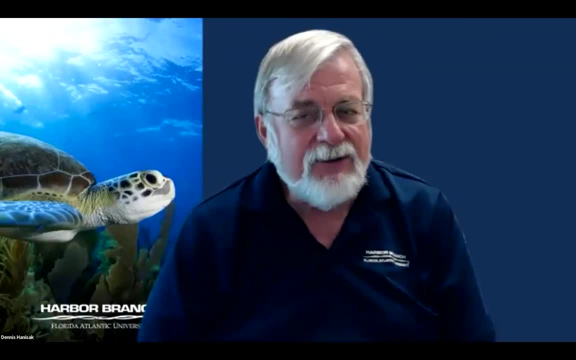 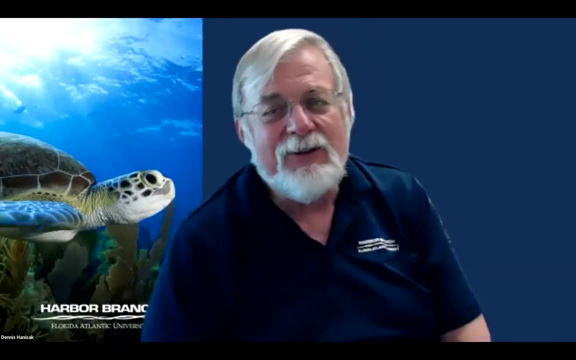 pretty, pretty pervasive. So I I guess yeah, for even exploration and tourism. Yeah, I think that's still a fundamental human activity, if you will. But when they went to study the giant squid, you know, being down there and seeing it was, was quite. 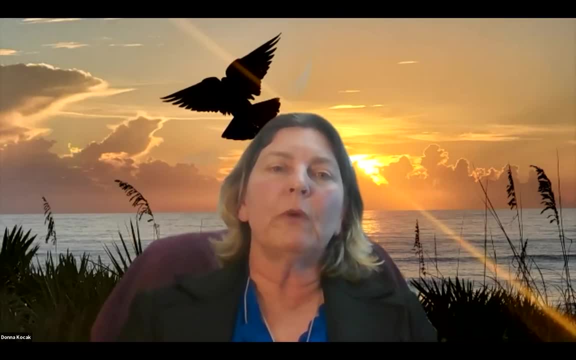 amazing. You know, they had the bioluminescent little attractor, jellyfish, And they got that on video. I mean, that was impressive too. But just being down there and seeing these things firsthand, I guess can mean so much to the scientists that study them for years. 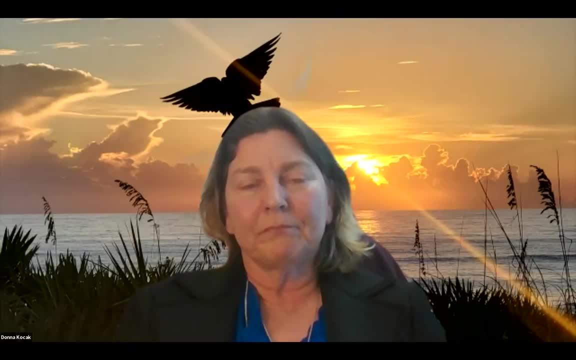 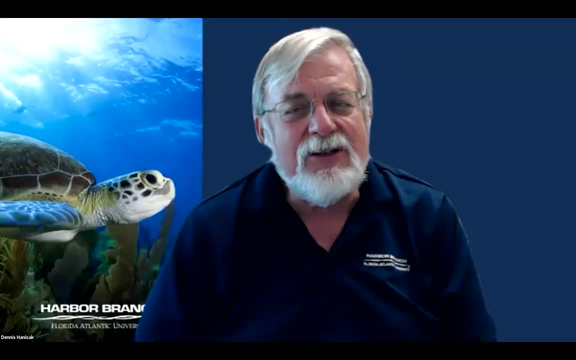 All right. well, I don't see any other questions coming in. So, Donna, before I thank you, is there anything else that you any other great vision or wisdom you see For ocean technology? that any kind of parting shots that you know our folks in the audience should kind of keep an eye?